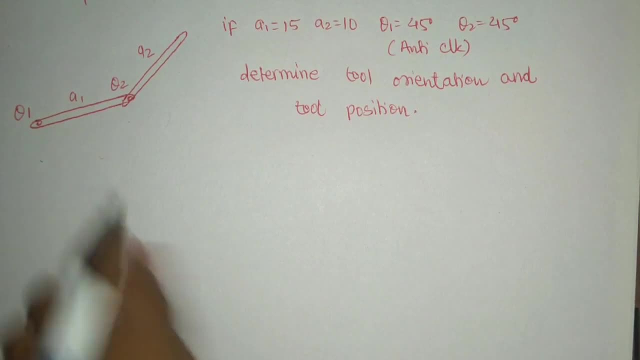 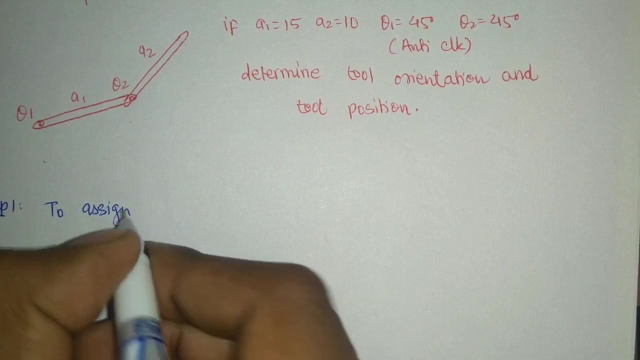 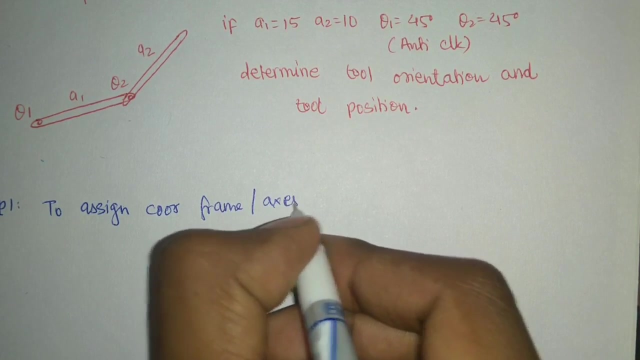 Now we are going to use the DH convention here. So the step one for DH convention is to assign the frame, to assign coordinate frame or the coordinate axis. So first of all, we are going to do that Now. in order to assign the coordinate frames, there are certain rules. 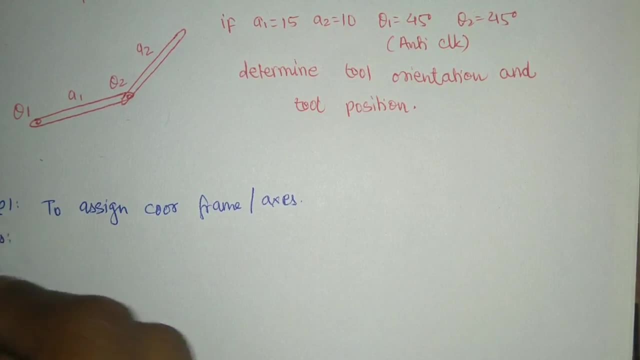 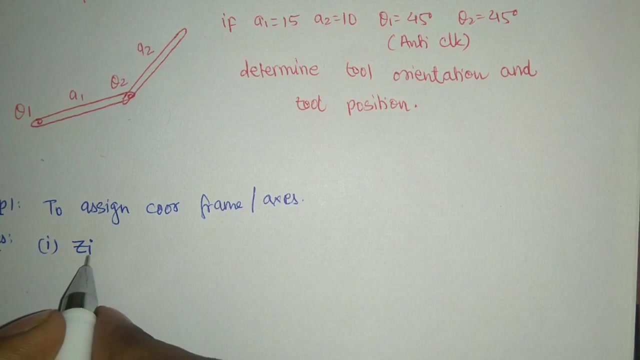 So the rules which govern the frame assignments number one is that Z axis, ZI. ZI means for any joint. we are going to use one axis or one origin over that one coordinate system for each of the joints. So ZI will be the joint axis. 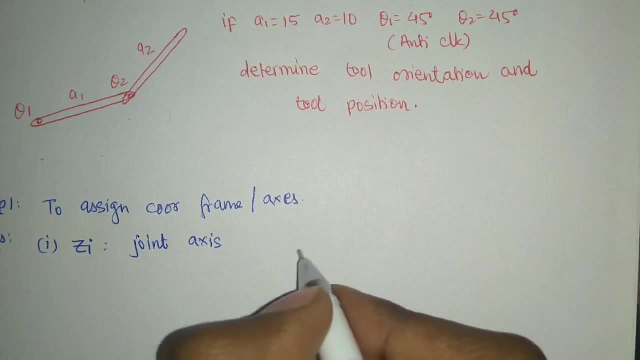 Now, what do we mean? A joint axis? joint axis is basically, if we are having a revolving system, right? So let us say, this is my link, which can revolve around this. okay, So the axis of this link is going to be perpendicular, or out of the paper or into the paper, right? 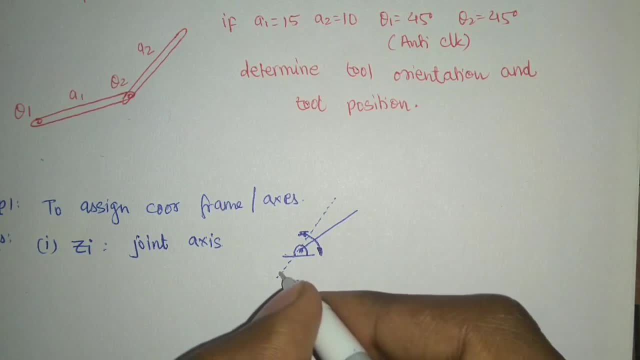 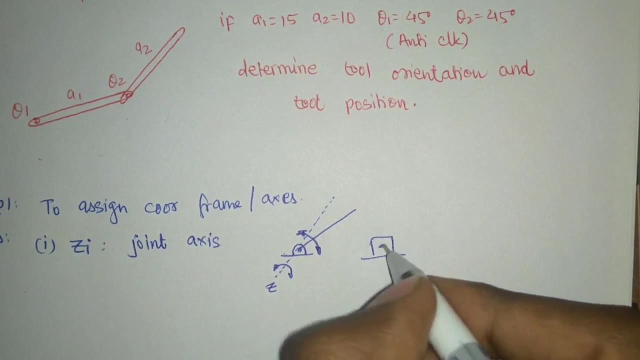 So this will be my axis about which it is basically rotating, right? So that is going to be my Z axis here. If it were a prismatic joint, okay, So in a prismatic joint, See, it can translate in this direction. 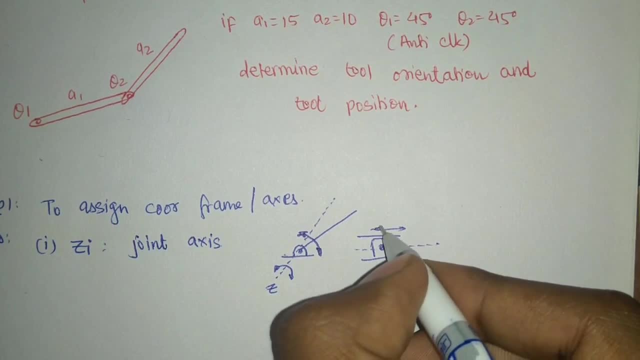 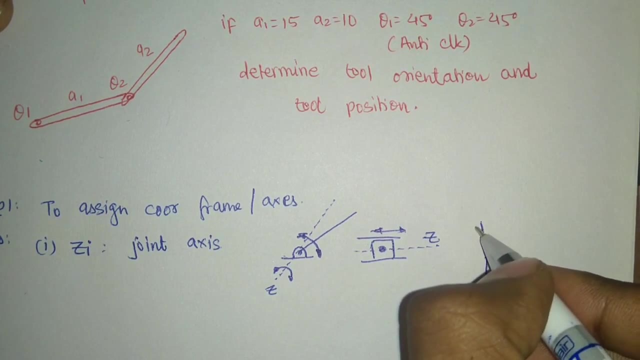 So this will, along, the translation itself will become my Z axis. okay, If it is very rotatory one, okay, revolving one, then let us say: this is my link, another link here, And now it can revolve around it, right? 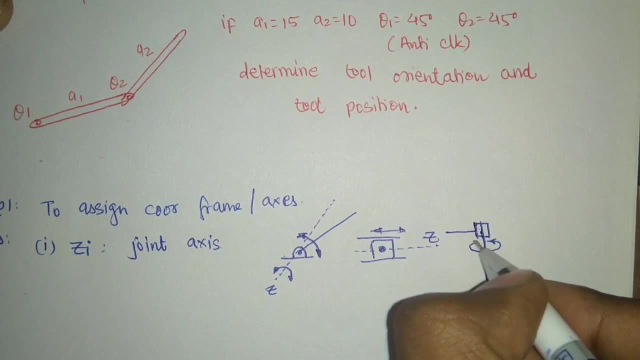 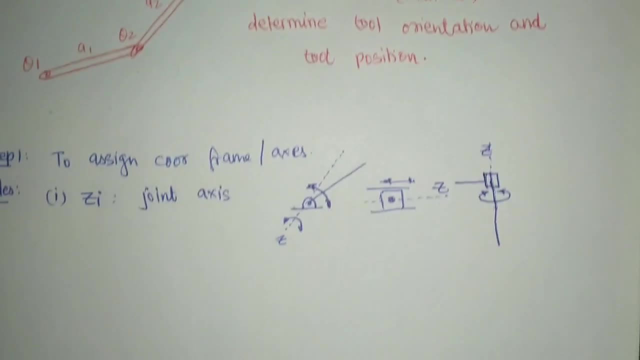 If it is possible to revolve it around this like this, then my Z axis would have been along this itself: okay, So that would have been my Z axis. That is how we define the Z axis, first of all. okay. 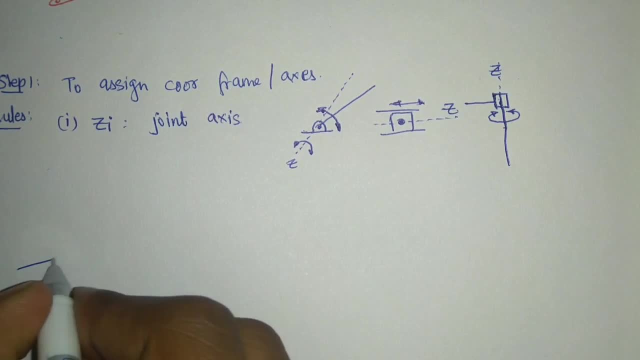 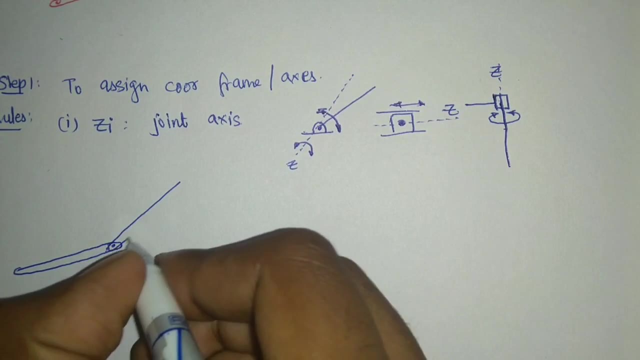 In this case means the two degree of freedom system that we are having over here. first of all, we are going to assign the this Z axis. okay, Now the assignment we do at the base, or we start from the first joint, okay. 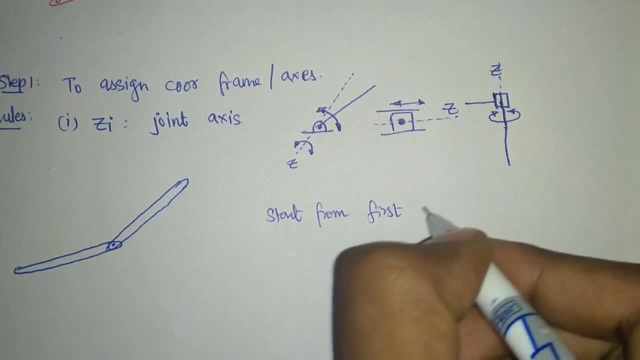 We start from first joint that we consider as our base right, And then go up to 2, okay. So whatever is the number of degrees of freedom, we will be assigning plus 1 to that, okay. So if it is possible to revolve around it, then let us say this is my Z axis. 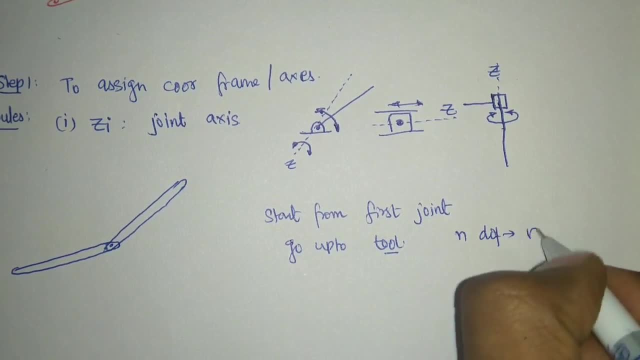 If here I am having n degrees of freedom, then I will be assigning n plus 1 frames, right? So in this case, since I am having 2 degree of freedom system, so I will be assigning 3 frames, basically, okay. 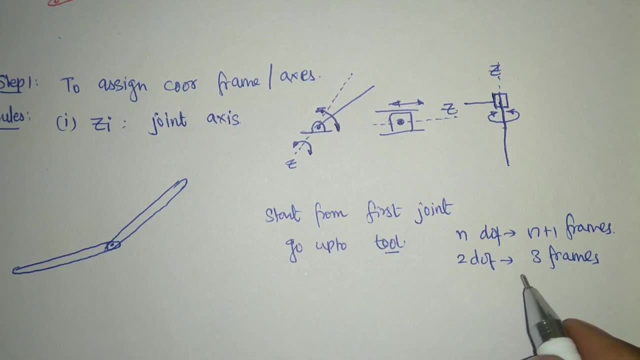 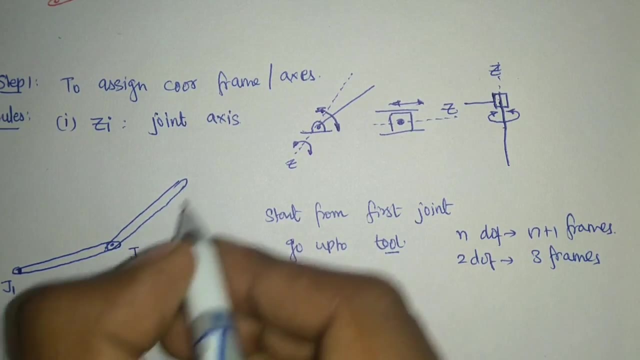 And these are moving frames, So our analysis will be based upon moving frame analysis only, okay. So here on this first joint, it is my joint 1,. this is my joint 2,. okay, And here is my tool, or my end effect, whatever I want to call it, okay. 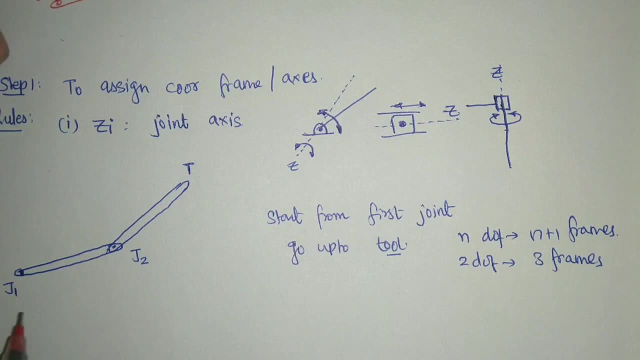 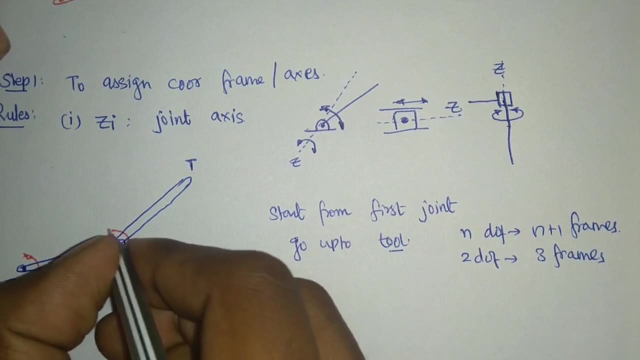 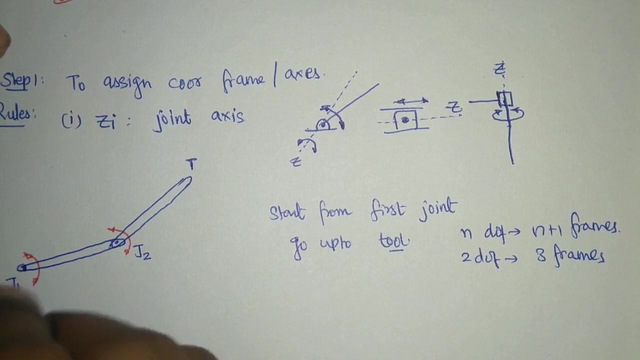 Now, what will happen here is That there is a rotation possible here. It is a rotation right. It can rotate around this And again it can have a rotation over here. Okay, and this is my tool. So here Z axis is going to be perpendicular to the plane out of the paper or into the paper. 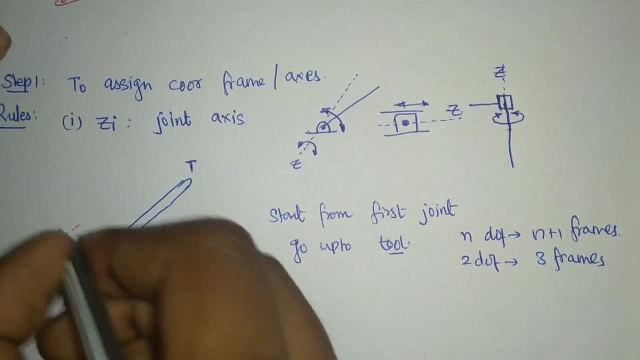 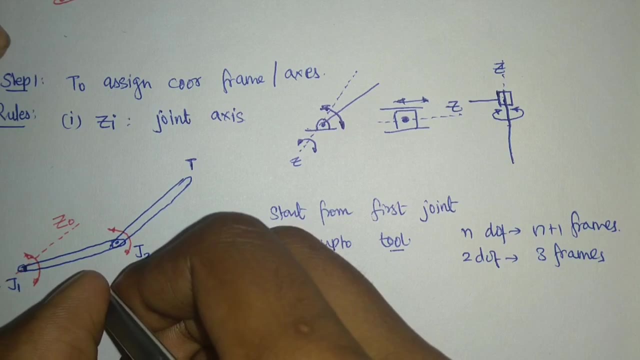 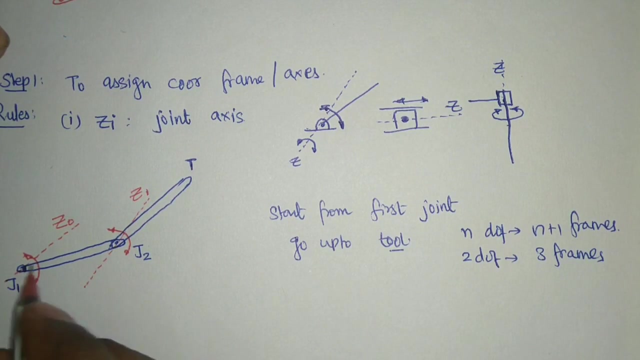 So let us say, this is my Z axis And this will be Z0.. I will start from Z0, right, Then second Z axis will be along its rotation here. Okay, So that will become my Z1.. And I have assigned these two Z axis based upon the joint function or the joint property. 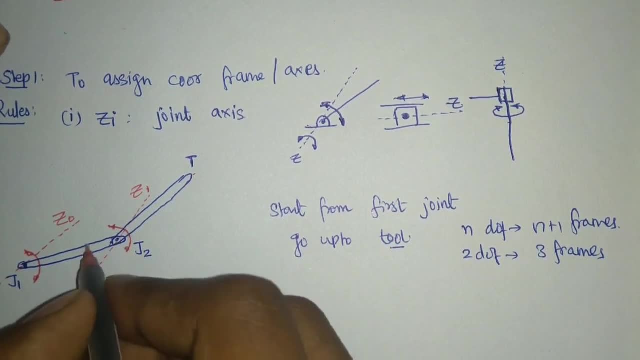 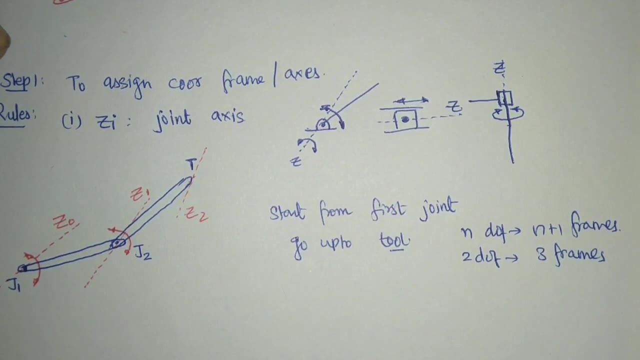 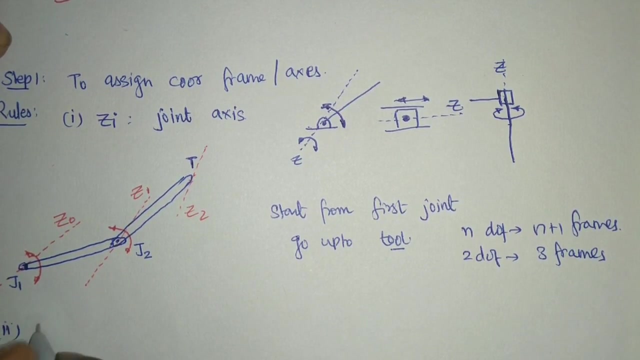 Now at the tool. I will simply put it same as its previous joint, which is joint 2.. So here let us say this is my Z2 for the tool. okay, So we have assigned the Z axis. Now the second step in assigning the frames is to assign XI or the origin. 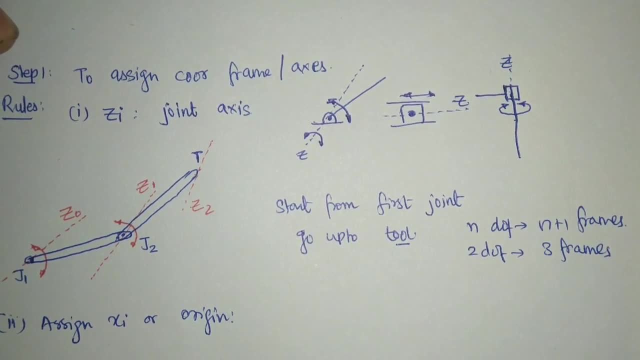 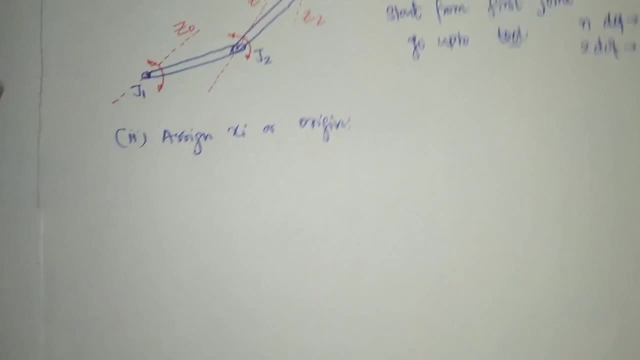 Both of these things we are going to assign over here Now. in order to assign our X axis or the origin, the one thing that we need to remember is that our X axis has to be perpendicular to ZI-1 and ZA. okay, 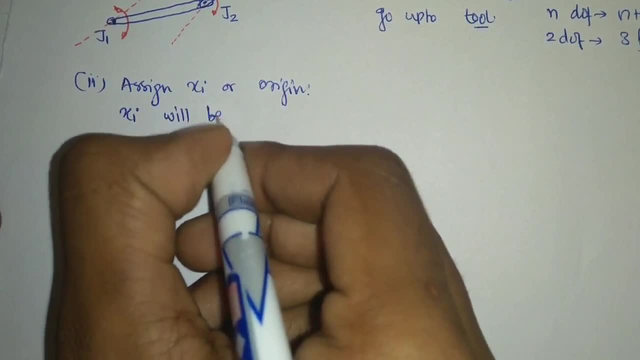 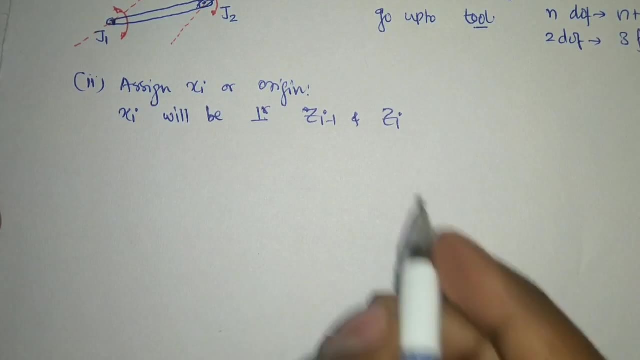 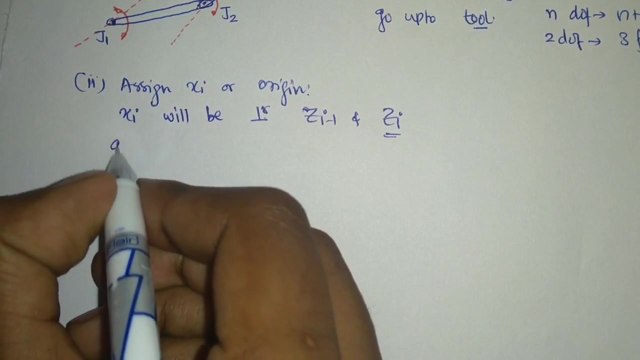 So XI will be chosen such that it will be perpendicular to ZI-1, and it will be naturally perpendicular to ZA, right, Because that is how we can assign any coordinate system here. Okay, So what I will do here is there are three conditions again possible here when I say ZI-1 and ZI. 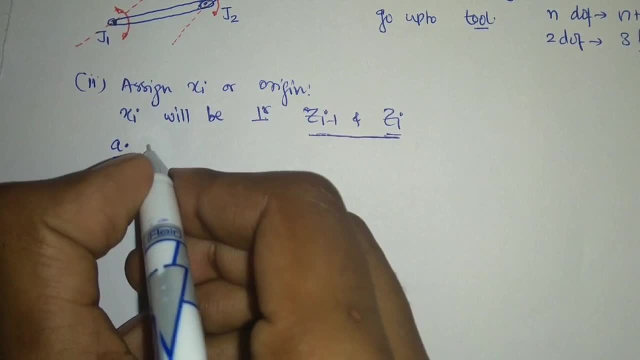 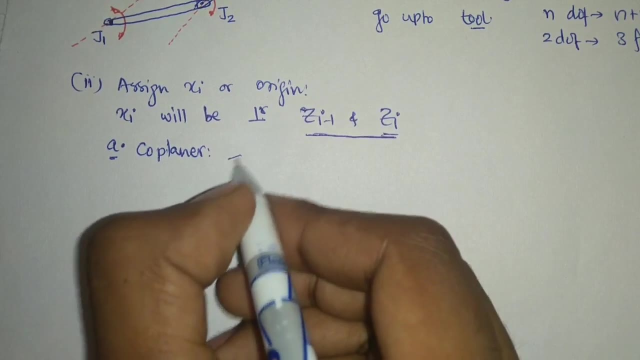 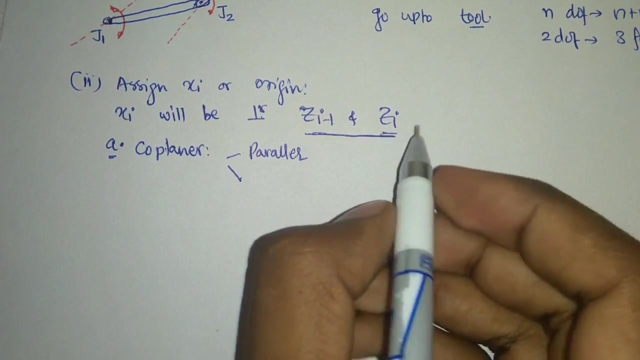 So one condition can be that these two are coplanar. Okay, They can be coplanar In coplanar. it can have again two conditions. one, that they are parallel to each other. Okay, So if ZI-1 and ZI are parallel to each other, the case that we are having over here- okay. 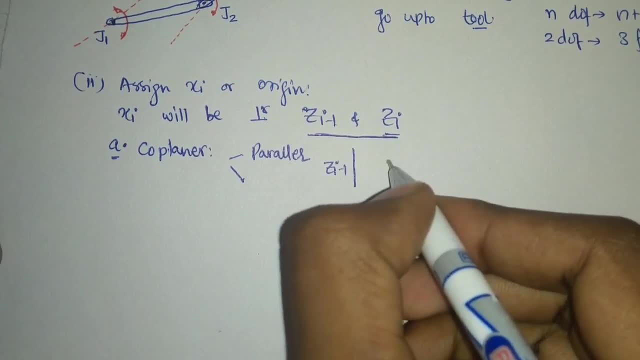 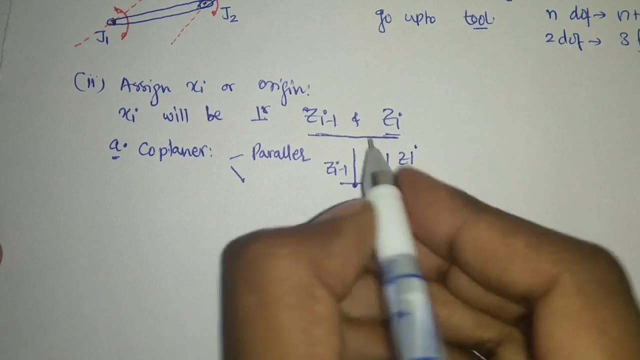 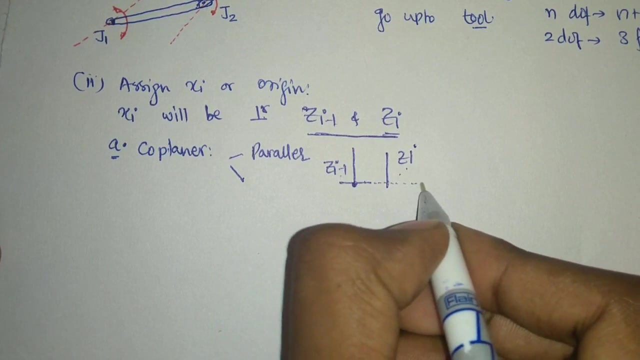 So in that case, let us say this was my ZI-1.. And this was my ZI. I have assigned these two and somewhere here it is having its origin. Okay, We have assigned the origin over here. Now to assign XI, what we do from ZI-1 to ZI. I will extend this line simply and this: 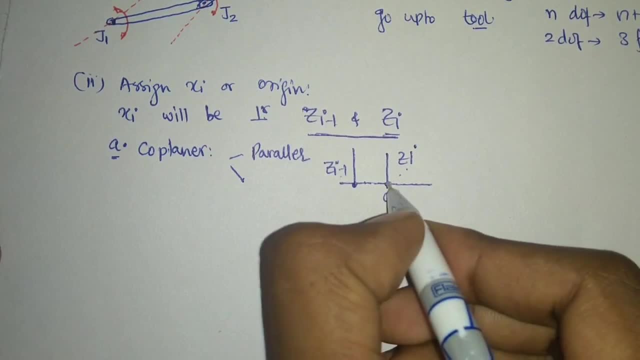 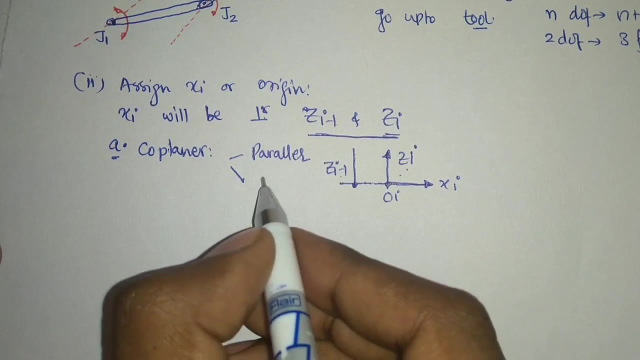 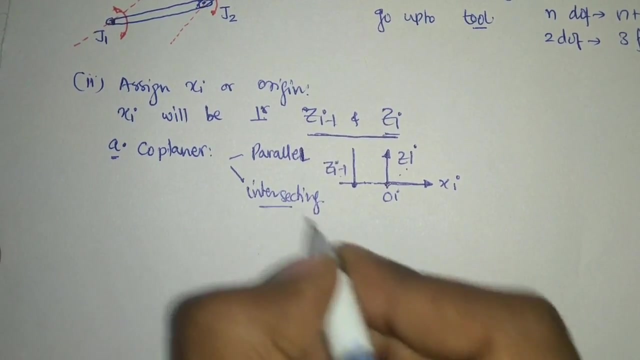 wherever it cuts it. that will give me the origin here and this line will become my X. Okay, Usually we use this one right Now. if it is not, parallel means they are intersecting, So they are coplanar. but they are intersecting, then whatever line which is perpendicular to 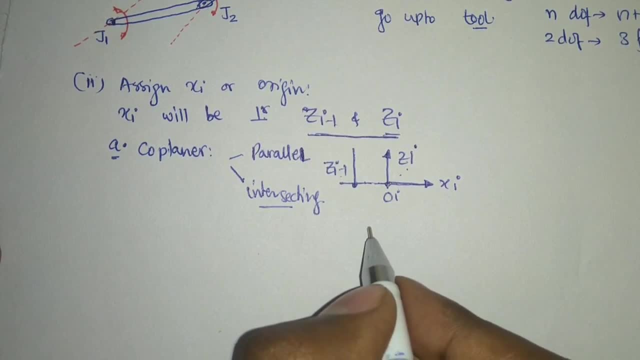 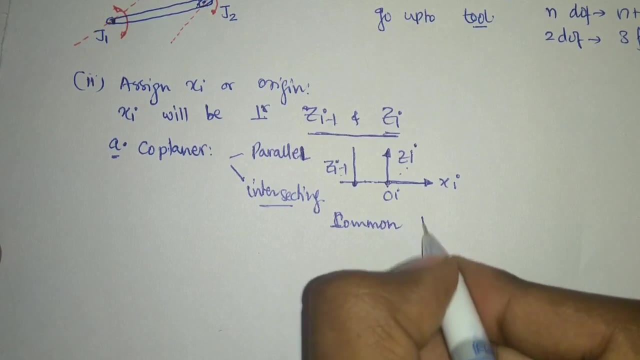 both of them. Okay, Since they will be intersecting each other. so there is going to be one line perpendicular to both of them, So common perpendicular. we will say, Okay, Common perpendicular, And from wherever they intersect each other that we can consider it as the origin. 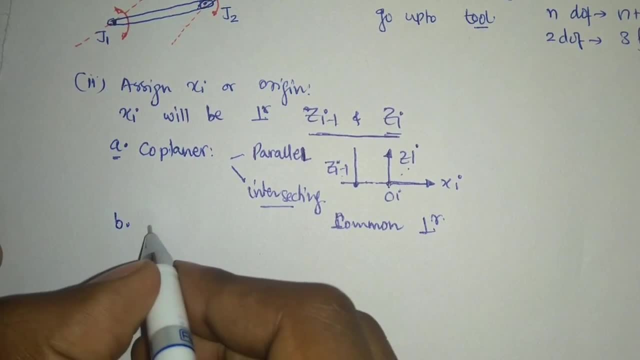 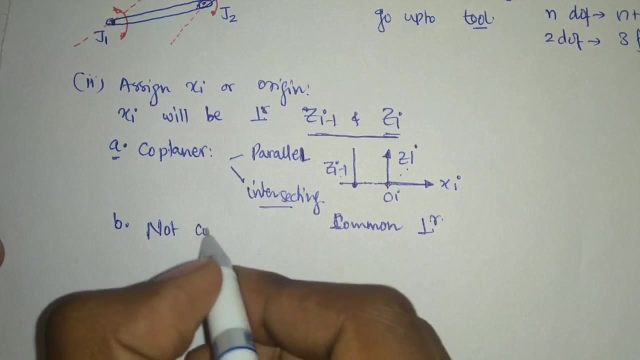 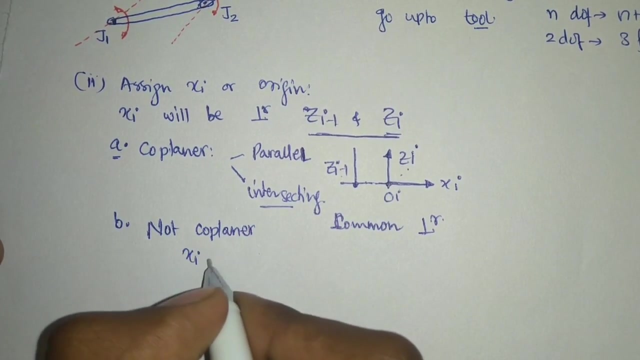 Okay, And we will make a common perpendicular from there. Now, second case: it can be that they are not coplanar. Okay, So they are not coplanar Now, when they are not coplanar to each other. in that case, what we will do? that XI will. 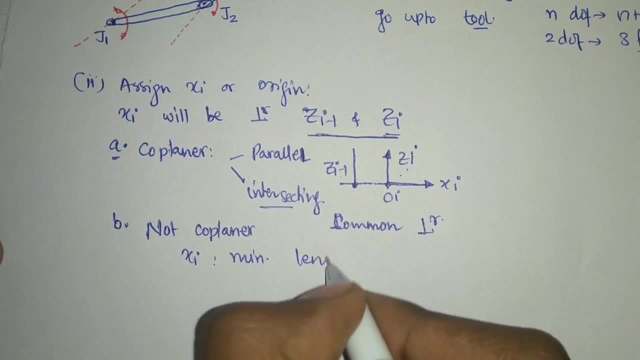 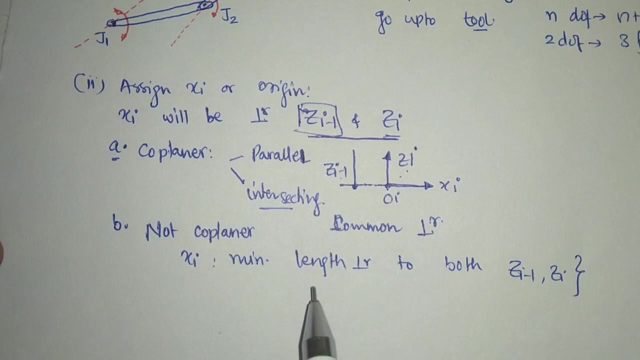 be represented by the minimum length perpendicular to both. Again, the perpendicularity has to be to both ZI-1 and ZI. Now, sometimes it may happen that we may not get the intersection with ZI-1.. Okay, Okay. 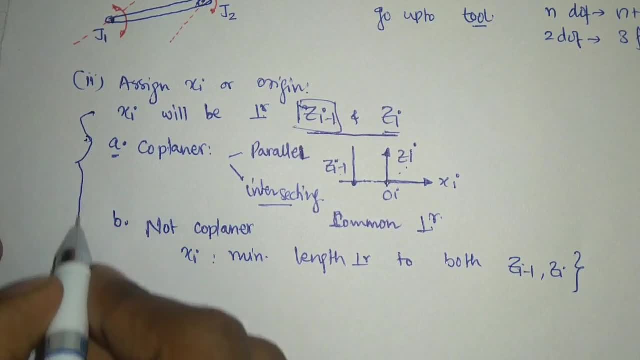 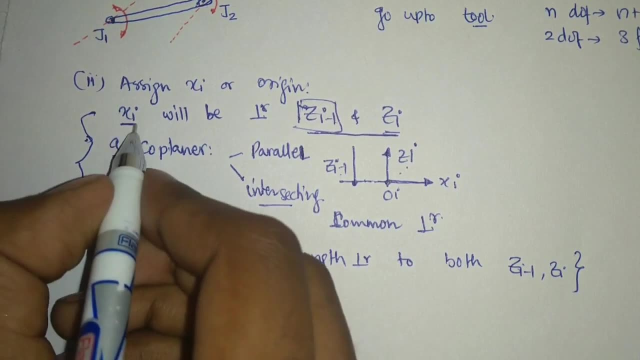 So let us talk about that later. Now to assign XI. these are our main rules. Now it is not necessary and it is not binding in which direction we take XI. XI is totally up to our decision. Okay, So we are free to choose the direction of XI. 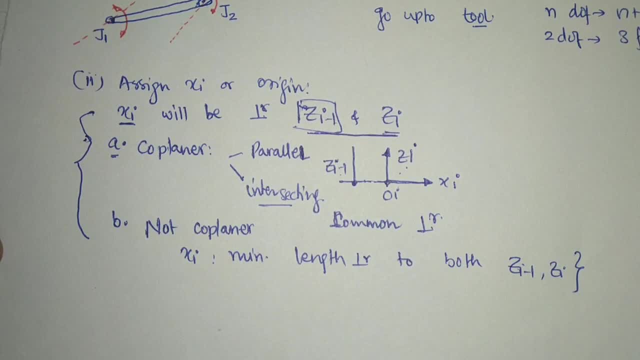 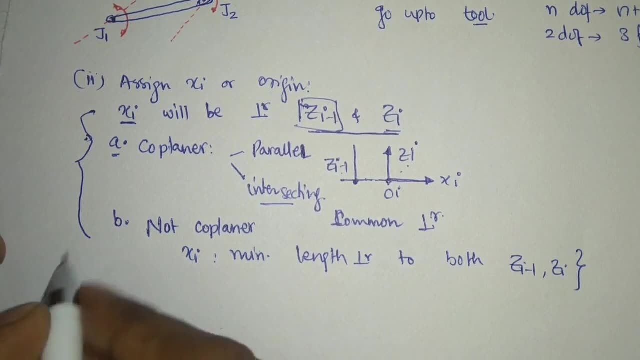 But we chose it such that we need to do minimum of the calculations Right. And those rules and those basically the thumb rules, we are going to discuss them again. Okay, Then the third rule to assign the axis would be: 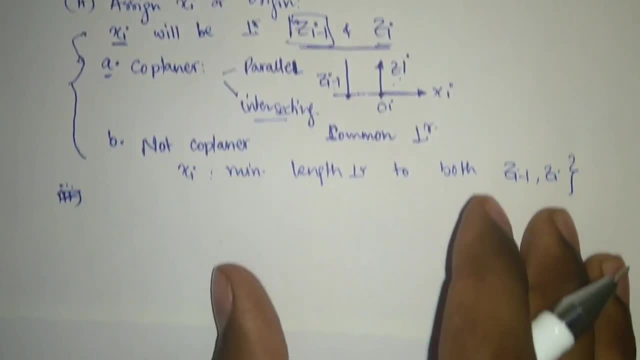 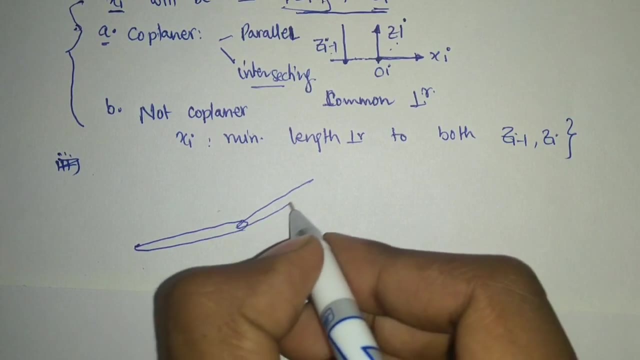 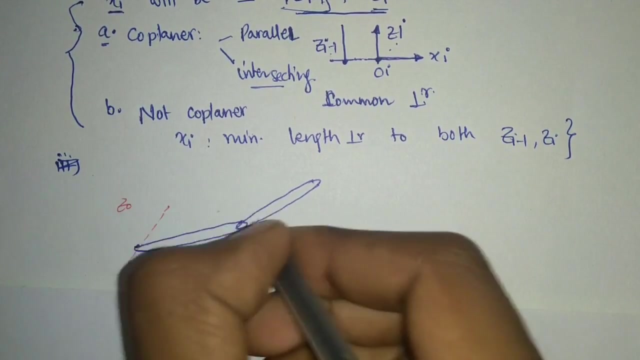 Okay, So let us assign the X axis here in our case. Okay, So this is my link 1 and this is my link 2.. Now I have already assigned Z axis. Right? This is my Z0, Z1 and Z2.. 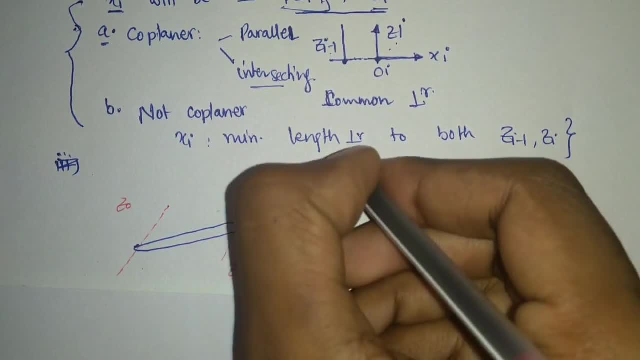 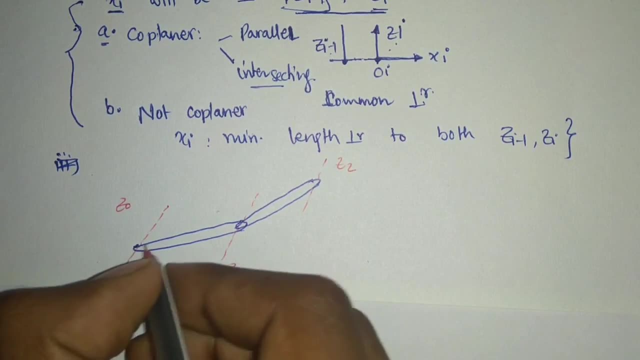 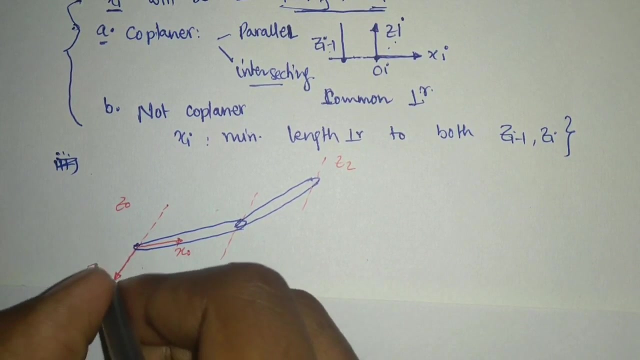 Now what I will do, since these two are parallel to each other, Okay, And in case of parallel now, okay, wherever I want I can put my X0.. Okay, So this is, let us say, my X0 and this is, let us say, my Z0, over here. 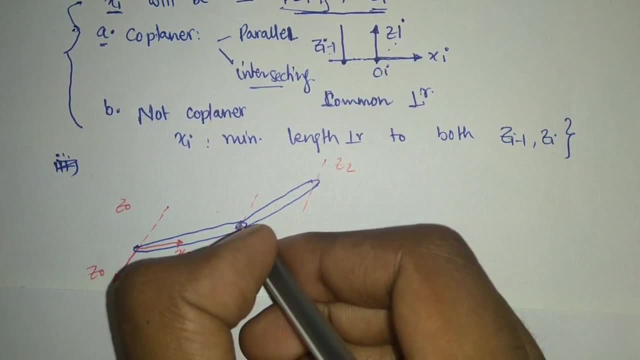 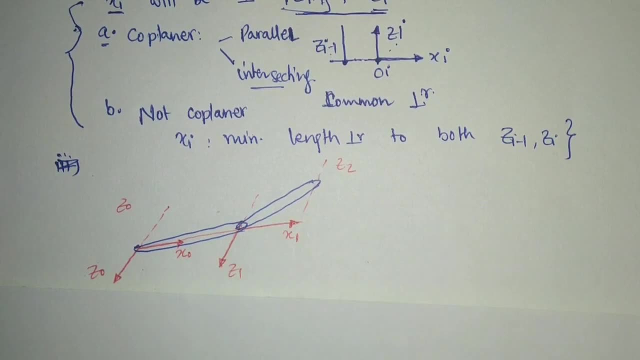 Okay, Now this will become my Z1 and I will put my X1, which will be along it. Okay, So that will become my X1.. Right, I have put Z1.. I have put Z2.. X1,, X2 and X0. 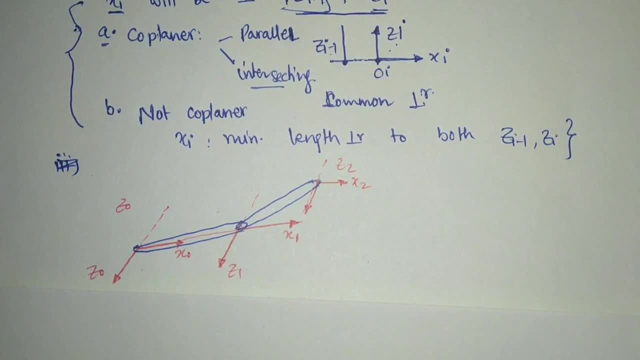 Okay So, X axis and Z axis. I have introduced onto this one. Okay, So, this is my Z1.. This is my Z2.. Okay, So, this is my Z1.. Okay, I have introduced onto this particular linkage. 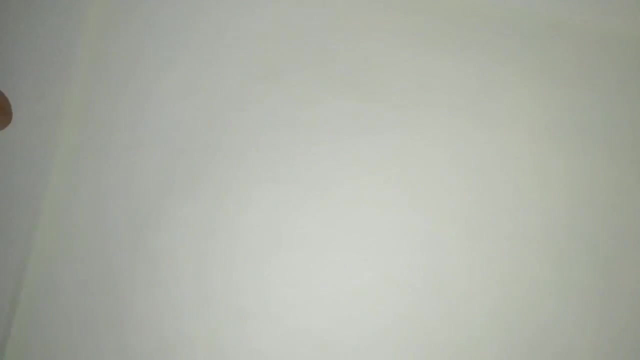 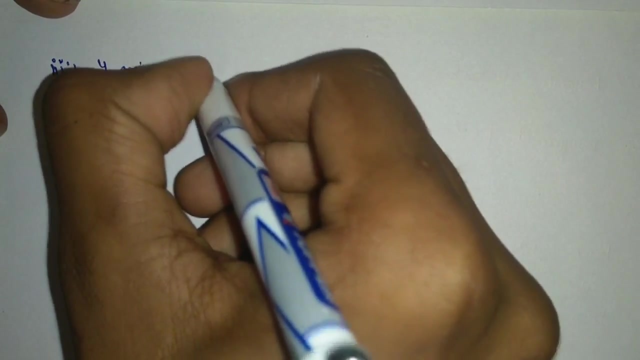 Now the third rule for frame assignment talks about the Y axis. Okay, Although when we have already assigned two axes to any frame, Y axis gets locked there because it has to follow the right-hand rule. Okay, So Y axis should follow right-hand rule. 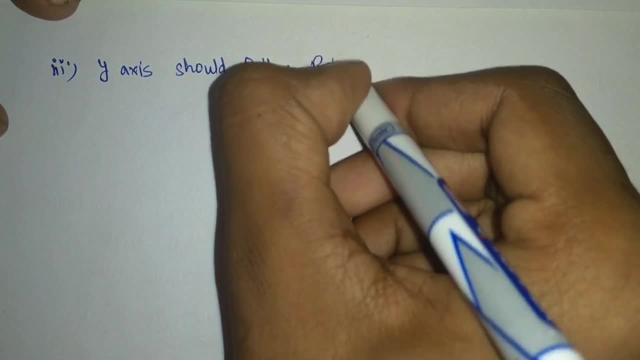 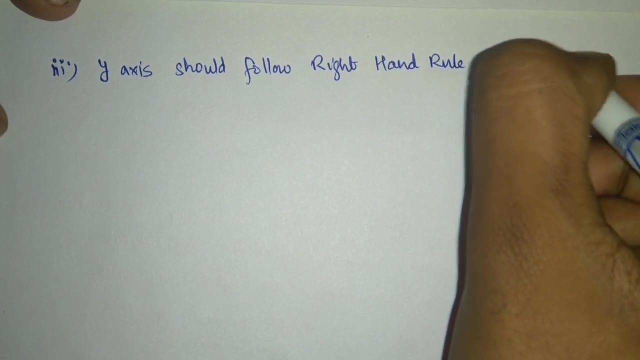 Right-hand rule. Okay, Right-hand rule. what is our right-hand rule? Right-hand rule is basically X. Okay. So basically, X- Y should give Z X. Y cross is Z, Then Z- X will give us Y. 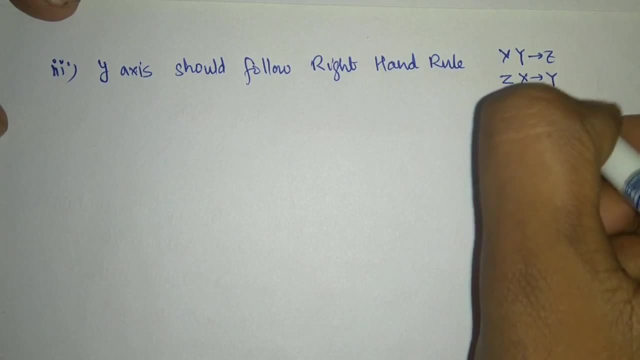 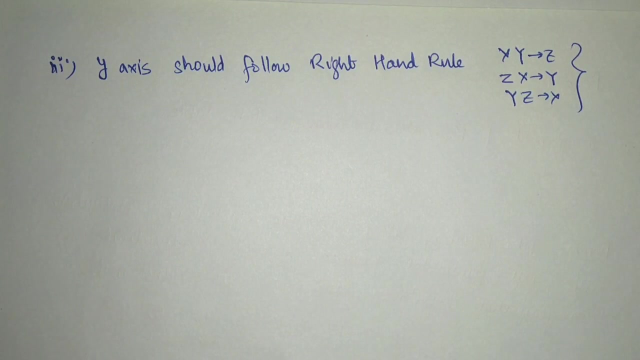 And then Y Z will give us X Right. That is our right-hand rule Cross-product basically Fine. So that should be followed by Y axis. But in our analysis, in our DH analysis, we will nowhere need Y axis. 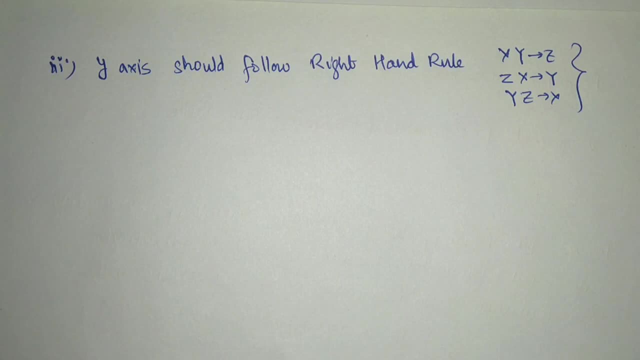 We will nowhere need the Y values, So we may, for the timing, ignore the Y axis here also. Okay, We do not need to put Y axis onto our this system. Now fourth rule: Now fourth is just a guideline here. 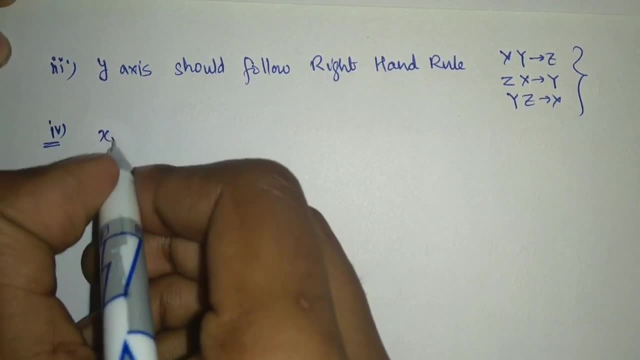 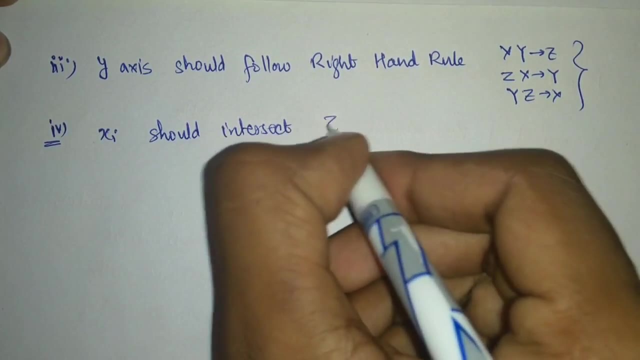 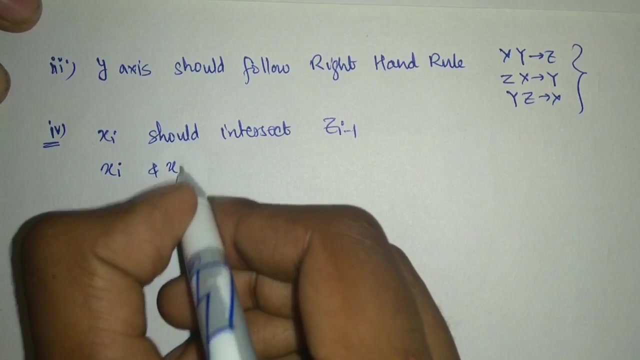 It is not a rule, basically, And it says that X? Y should intersect Z Y minus 1.. Okay, Z Y minus 1 should intersect here. And one more thing is that it will be good if X Y and X Y minus 1 have zero angle. 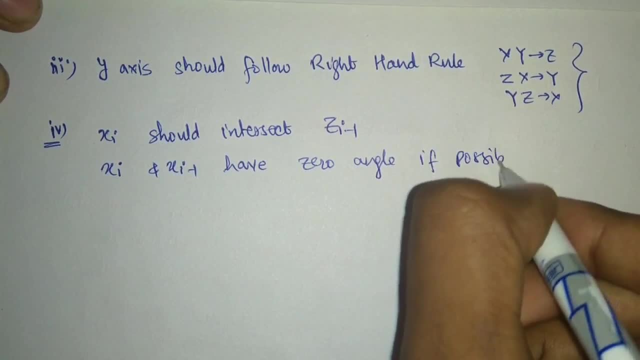 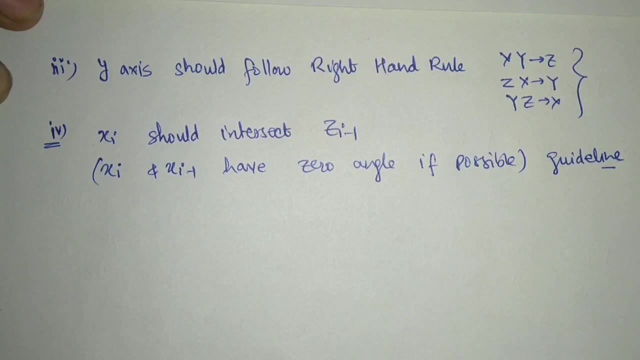 If possible. Okay, It is just a guideline. Okay, It is just a guideline. This is not fixed. It is just a guideline here. It is not a rule. It is just to ease out our calculations, Nothing else, Okay. 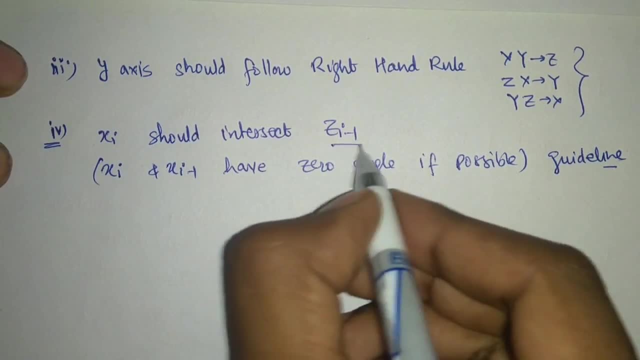 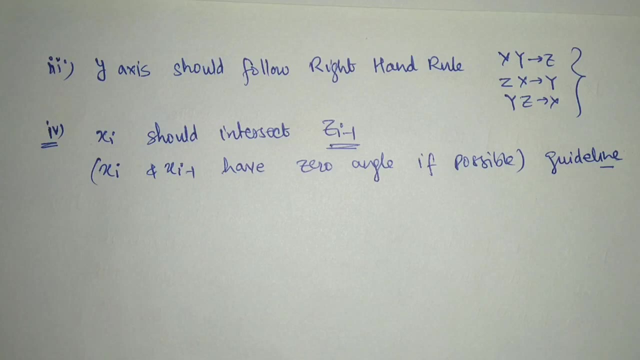 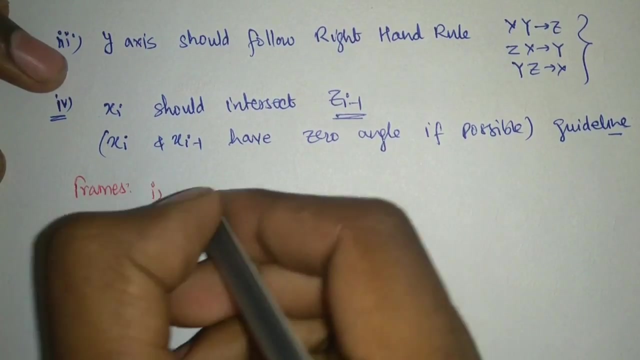 Now, in case it is not possible, then it is not necessary that we put our, these joint or our frames onto the link end. Okay, So the conditions for these frames is that frames number 1, they are rigidly attached to the link. 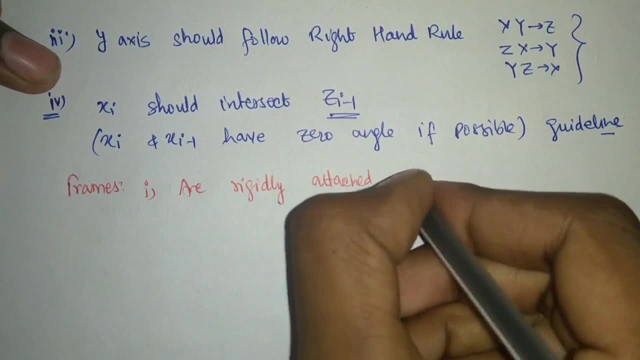 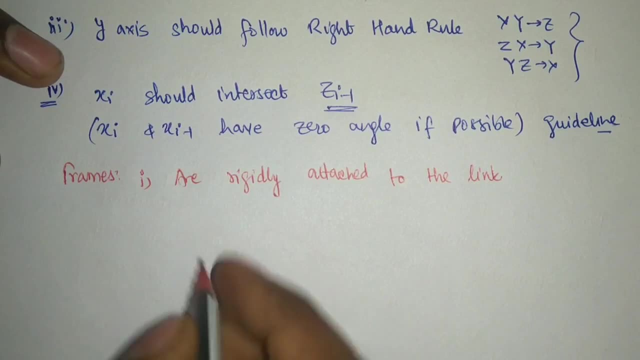 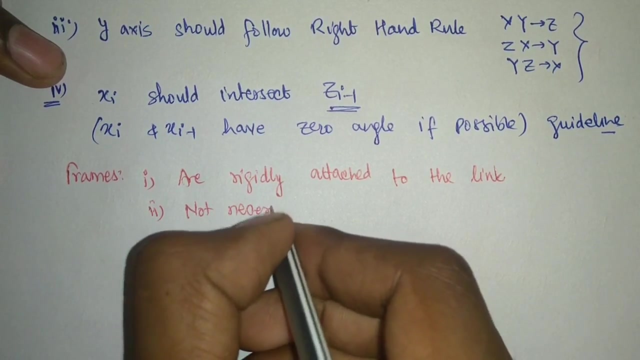 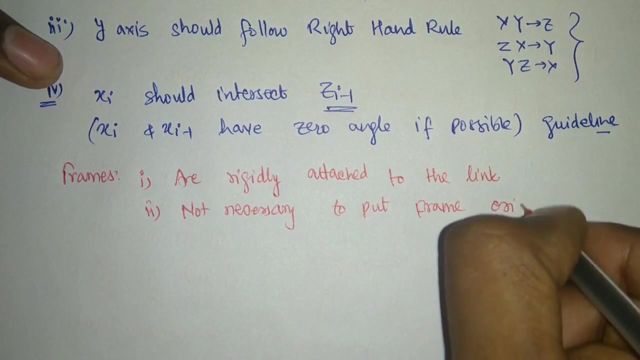 That is the one condition. So we are not bothered about their position, exactly because it is anyways going to have same sort of motion or movement. And second point: is not necessary to put the frames or to put the frame origin, frame origin on link end. 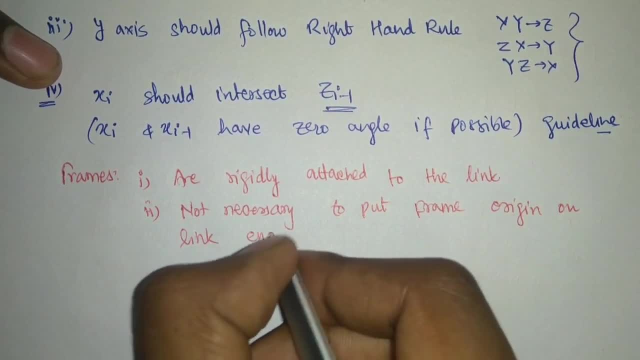 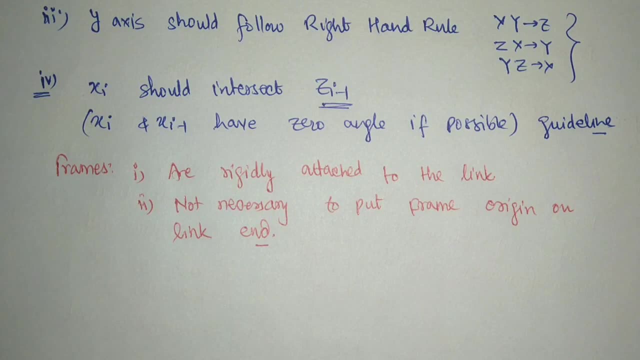 Okay, So it is not necessary that we put them onto the link end. Okay, So it is not necessary that we put them on the link end. We can have the origin and the frame at any location. It has to be just as per. the z-axis has to be as per the joint and x-axis has to be as. 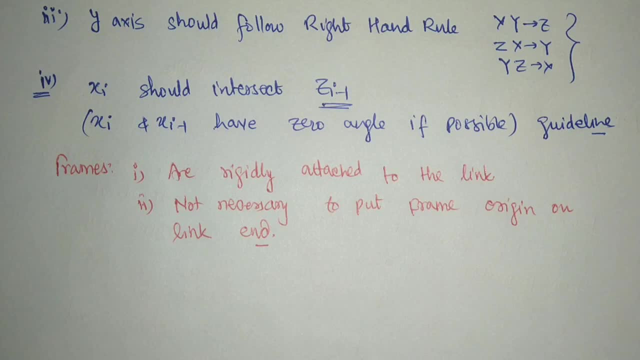 per the 2-3 guidelines that we have just laid out here. Okay, So in our case, we have already explained the z-axis and x-axis. Now let us move to the next step, and the step number 2 is to identify. to identify: 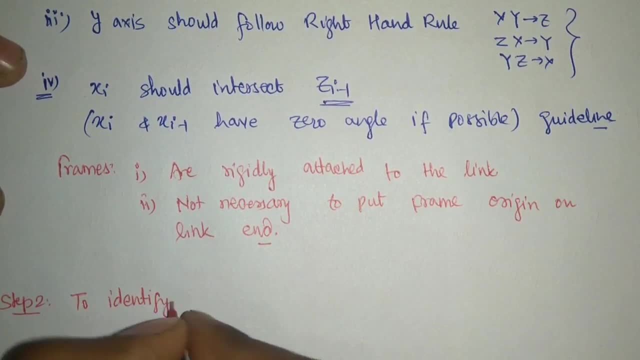 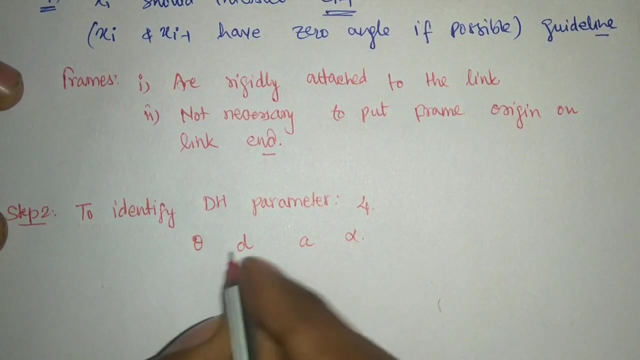 D-H parameters. Okay, So whatever D-H parameters we have over here, we need to identify them. And how many D-H parameters are there? There are four D-H parameters, namely theta, d a and alpha. Okay, Now, what are these and how do we identify them? 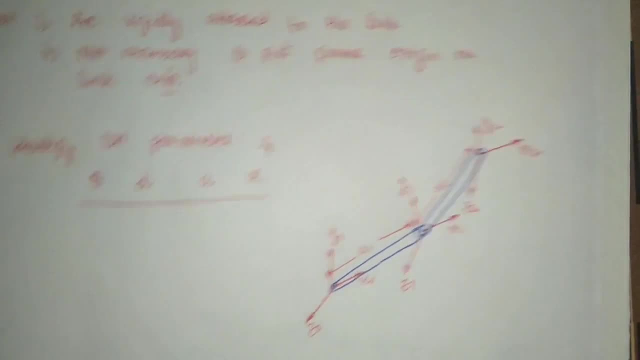 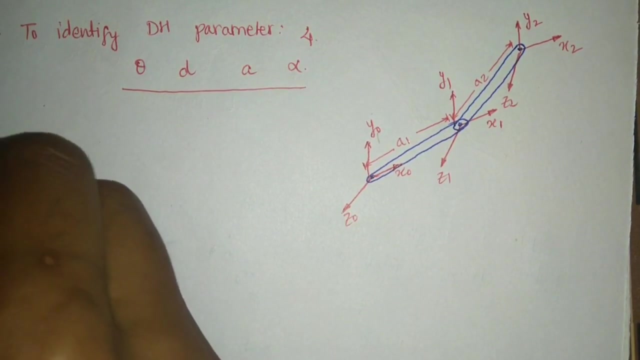 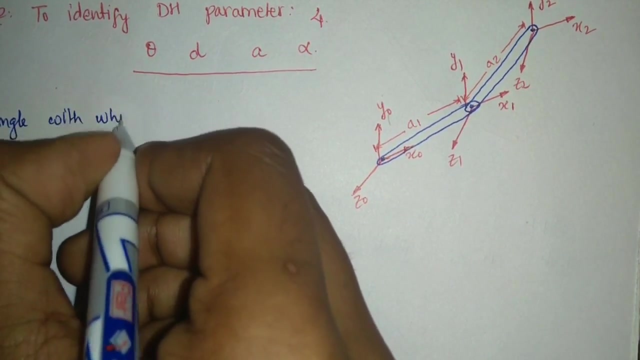 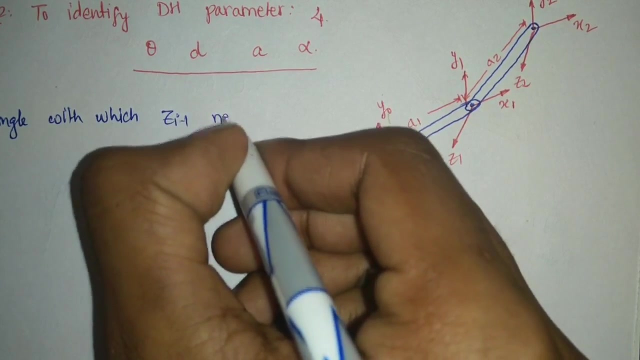 Let us discuss that. Okay, So let us identify these parameters. So first discuss what exactly are those parameters? Okay, okay, so theta, it is basically the angle with which, the angle with which we need to rotate our zi minus 1. okay, with which zi minus 1 needs to be rotated? I am 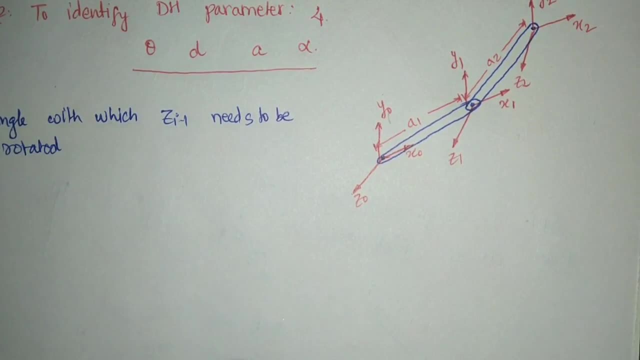 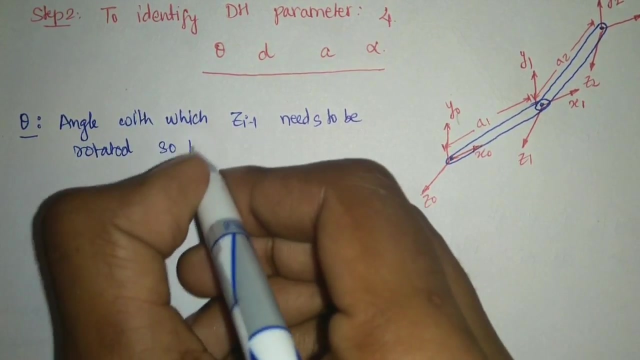 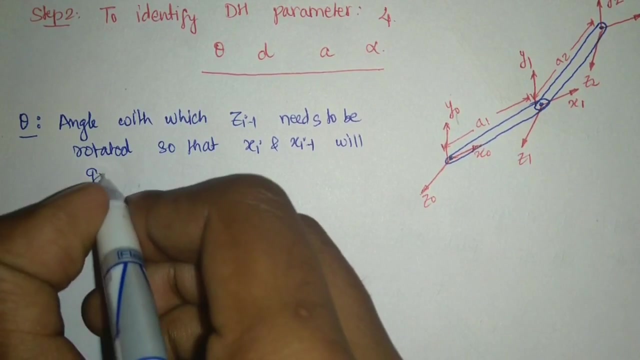 taking a lot of time here so that you understand the concept. in later on we can just take up, pick up our space there. okay so angle with which zi minus 1 needs to be rotated so that xi and xi minus 1 will get aligned. okay so they will get aligned with. 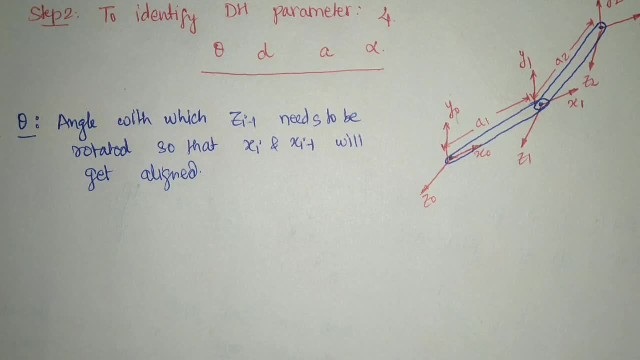 each other, or basically they will get parallel to each other, so that in that manner we need to this, we need to rotate the zi minus 1 axis. okay, so that is our basically theta. then the second thing that we have over here is d. d is the. 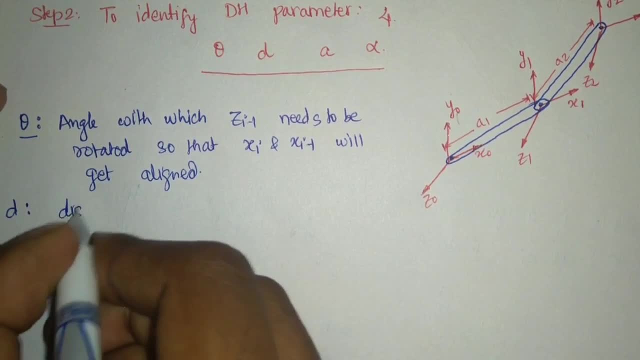 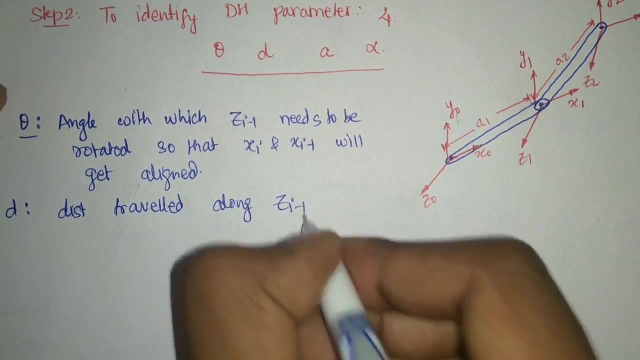 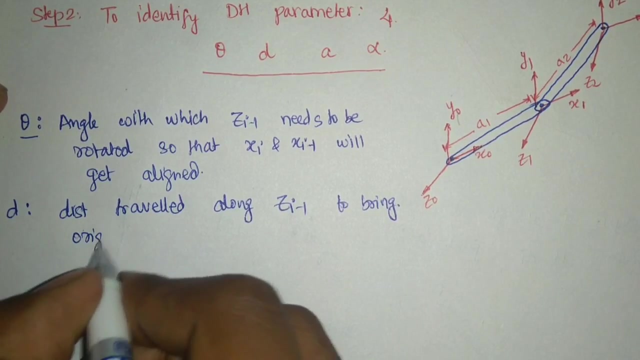 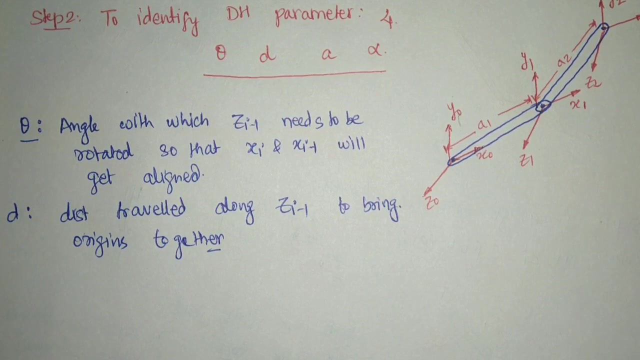 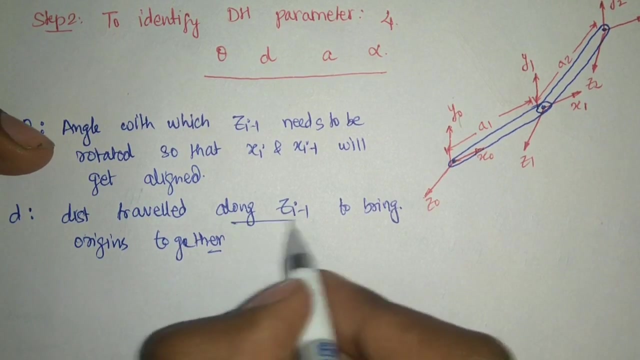 distance: okay, so distance traveled along, traveled along zi minus 1 axis. okay, zi minus 1 axis. to bring origins together? okay, origins together in order to bring the two origins together. basically, how much distance we need to travel along the z axis? okay, it is important here, along the z axis, that distance may. 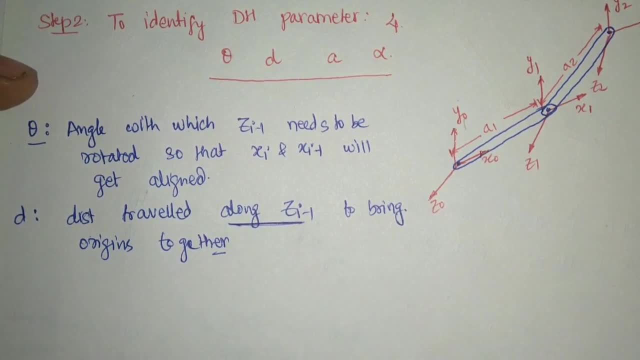 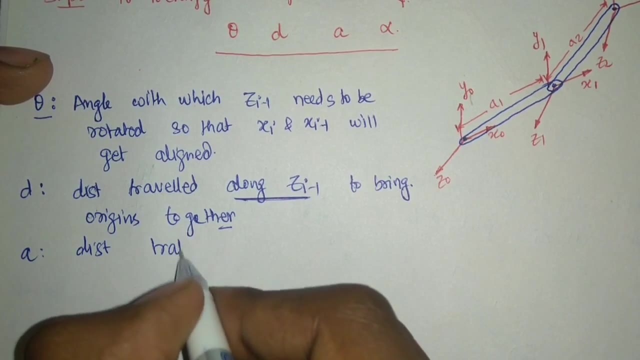 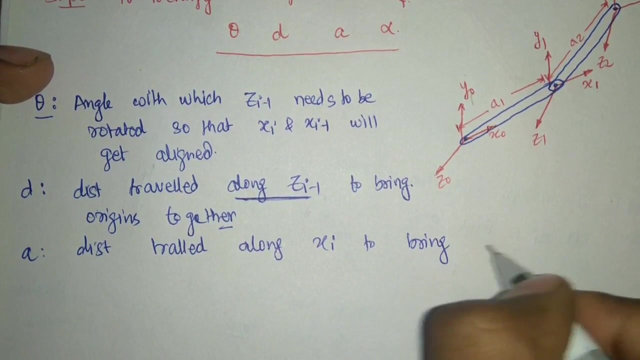 be zero in some cases, that we are going to discuss it, all the parameters we are going to discuss, okay. that third one is A and a is the distance travelled along. xi. okay to bring origins together or in line with each other. whatever is the possibility, we will do that, okay, maybe. 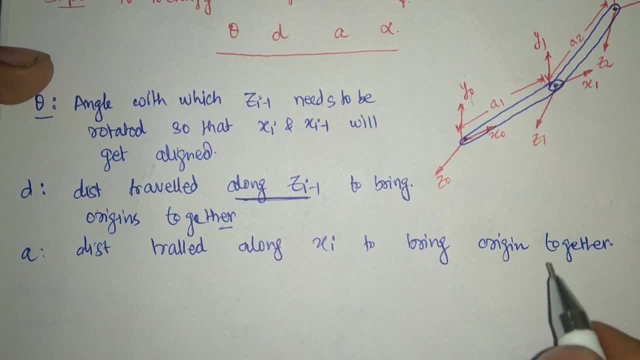 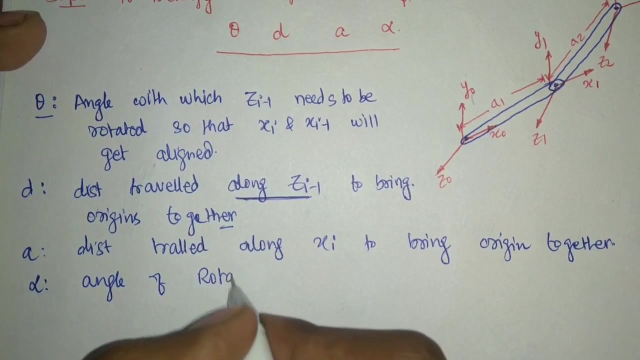 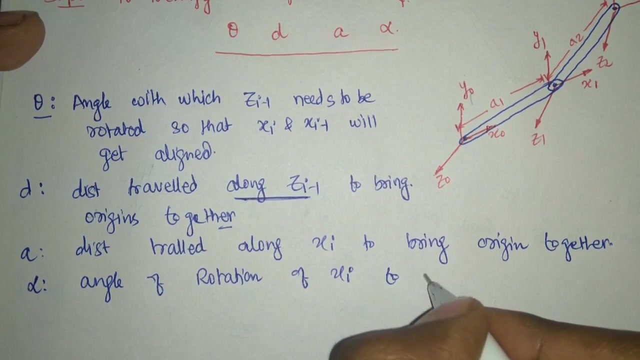 not at the same point, because it may not not be possible to bring them at the same point by moving along x-axis, so whatever is the nearest or the closest distance that we can have to them. okay then a alpha is angle of rotation of xi. after along xi to a line, zi minus 1 and z. okay, so such will. 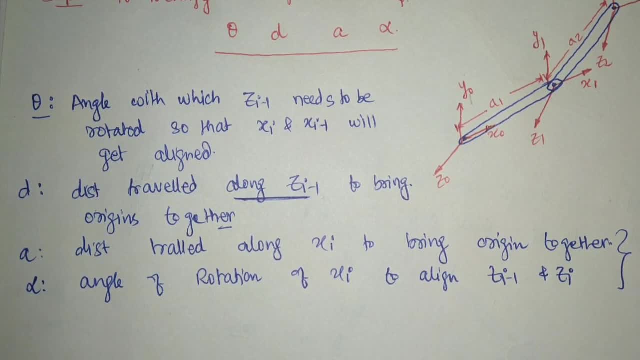 be our these requirements for all the four parameters that we have now. when we talk about the dh convention, there is one question usually asked: why do we actually use dh when we are already having some graphical method and so on? so dh is converting all. 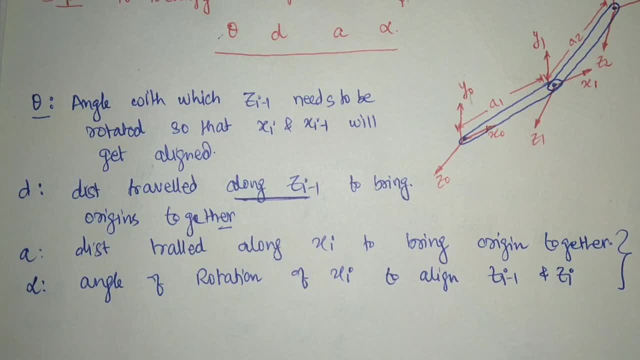 our analysis into these four parameters only. okay, so it is basically simplifying our analysis. we need not give it that much time as we would have given in graphical method. okay, this is a 2 degree of freedom. that's why dh may seem a little bit too much, but it is a 2. 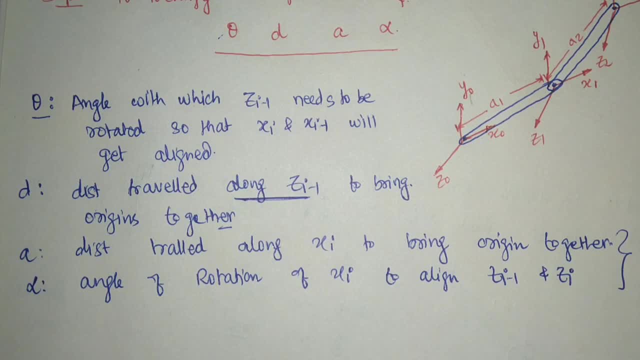 degree of freedom. that's why dh may seem a little bit too much, but it is a 2 degree of freedom. graphical is too easy here, but when we are having complex robotic systems or maybe 4 degree or 5 degree of freedom system, then it is always better to use dh parameters. 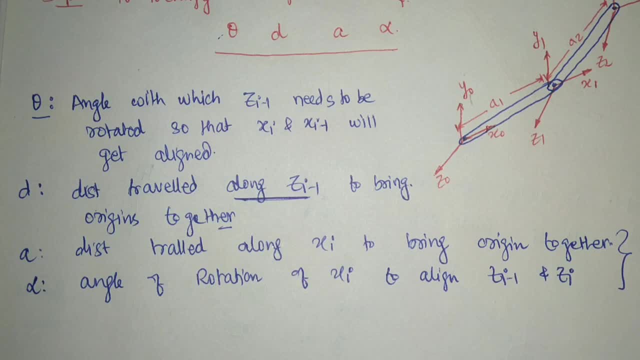 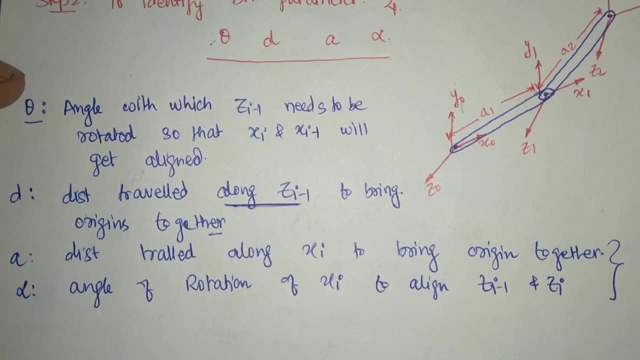 because graphical will not work there at all. okay, now let us see the values of theta, d, a and alpha for this system that we are having over here. okay, so third step is to make the table. okay, so step 3.. 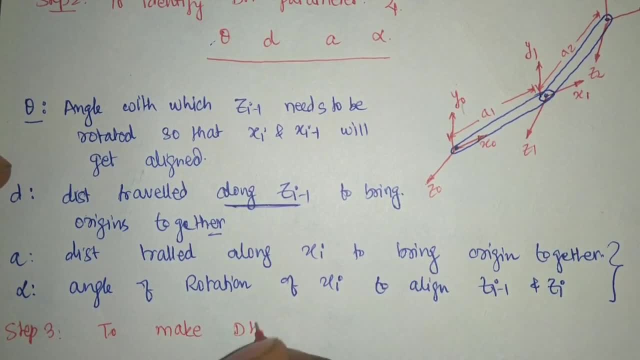 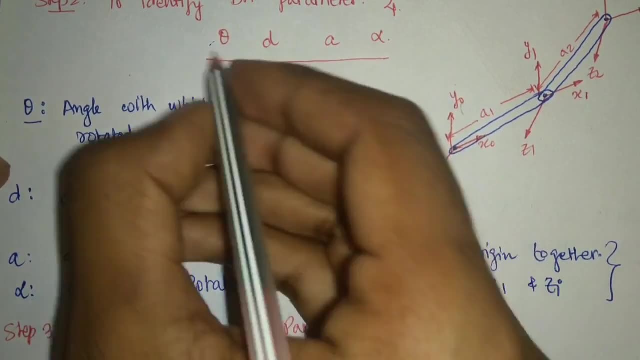 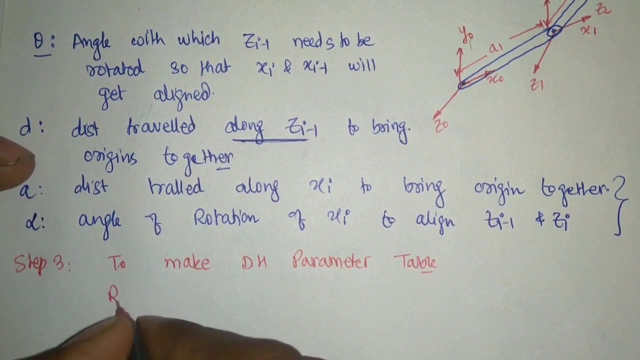 To make dh parameter table: dh parameter table. okay, now, in order to make the parameter table, what we need to do is we need to identify all these things and we need to know how many number of rows and how many number of columns that table is going to have. okay, so, number. 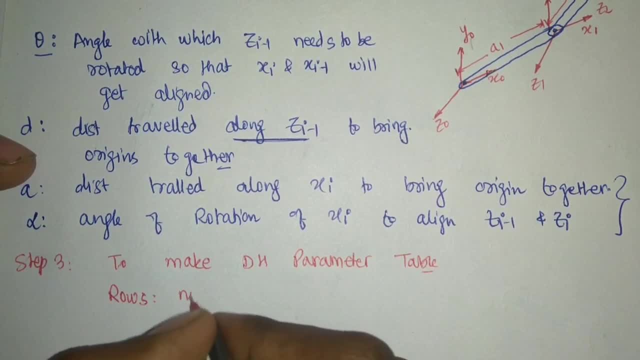 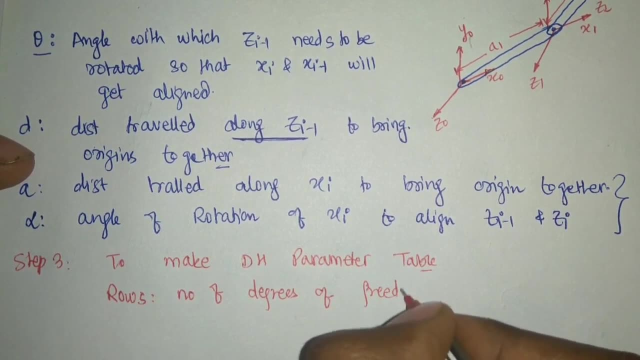 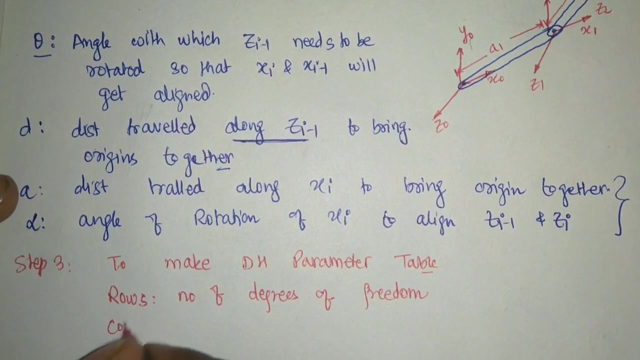 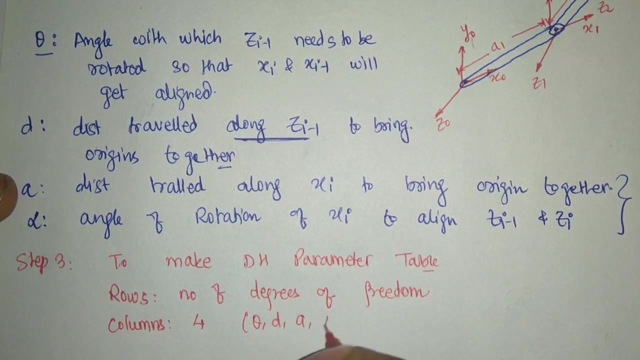 of rows in that column will always be equal to number of degrees of freedom. okay, so n? n, it is always going to be, and this number of columns, number of columns, will always be equal to 4, that is all those 4 parameters, only theta, d, a and alpha. okay. 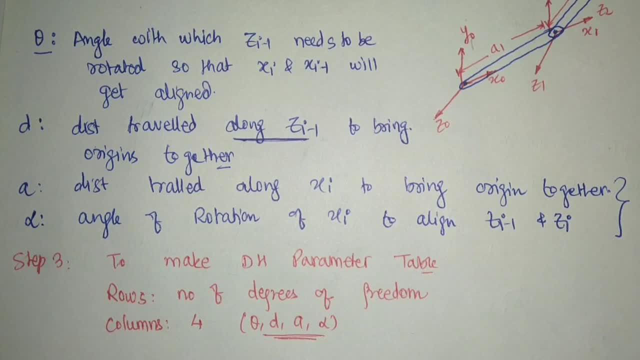 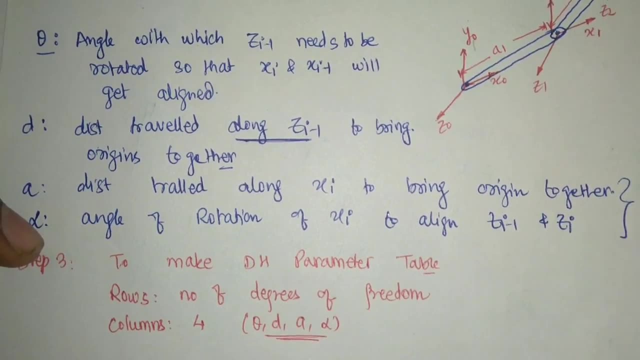 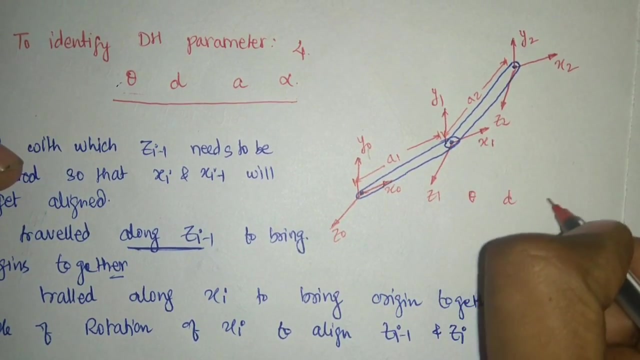 that is what we basically mean over here. okay, now let us determine those parameters here and have a look at it. see, in this case, okay, so this is the number of columns. okay, I am having theta d a. I am making it here so that we can look at the chart and the table. 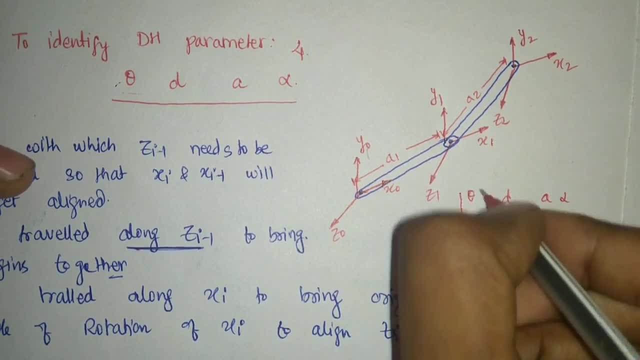 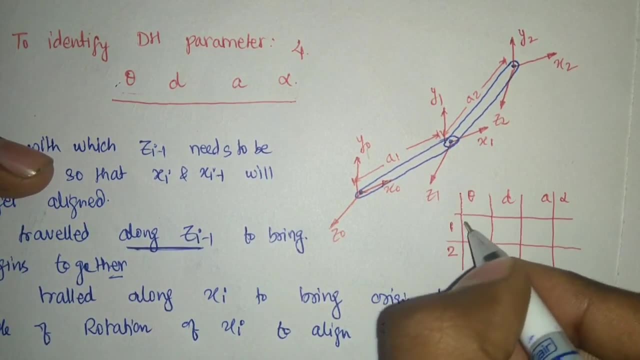 constantly 1 and 2, because I am having 2 degrees of freedom, right, okay now. first one is that theta. so 1 is going to represent between z0 and z1,. okay, so theta1 will basically be representing between z0 and z1. 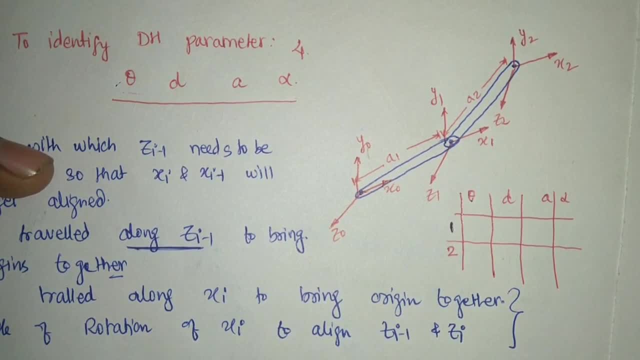 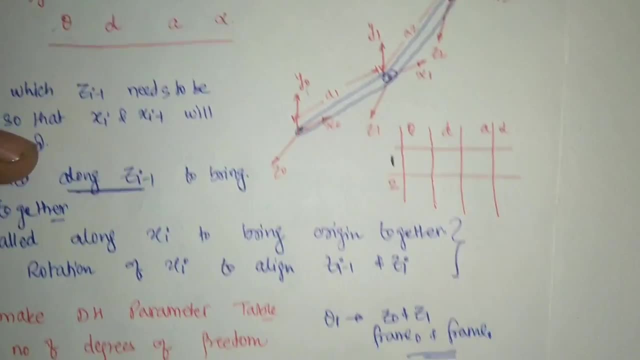 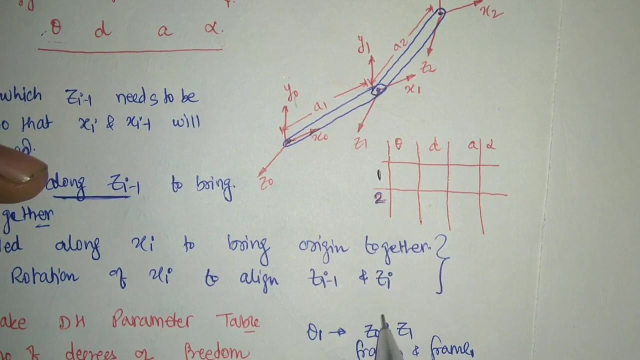 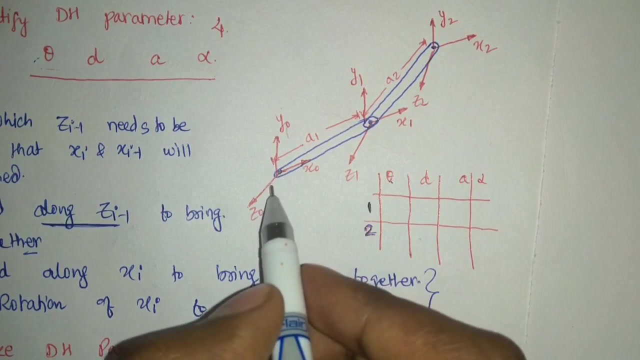 Okay, Or basically the frame frame 0 and frame 1, okay, that will be sorry. yeah, that will be my one number here. 2 will be representing between 2, frame number 1 and frame number 2, okay, so let us do it here. theta is the angle with which we need to rotate z0, so that 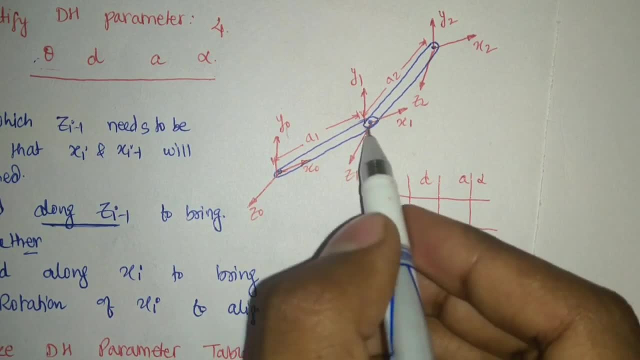 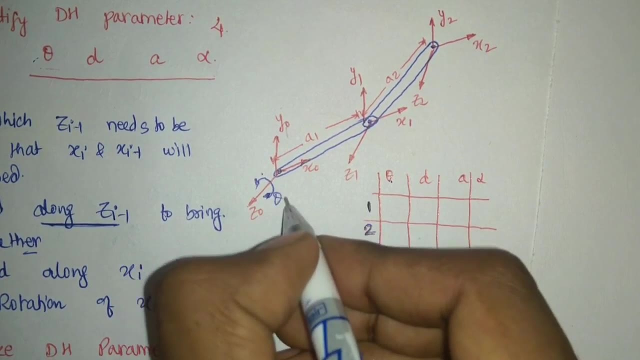 x will get parallel to each other. okay now, x will get parallel to each other. okay, so x will get parallel to each other, since there were a possibility of rotation- theta0, theta1 here- right, it could have rotated with theta1, so that is the angle that we need to rotate. 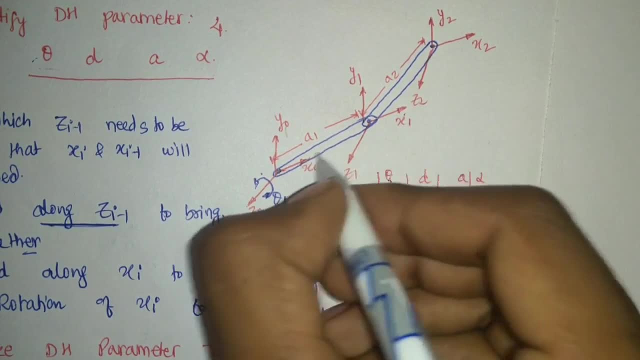 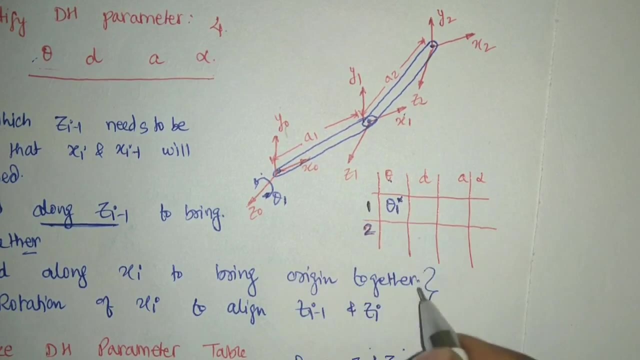 z0 with, so that x1 and x0, they will get parallel to each other. okay, anyways, wherever we have the joint parameter, we simply write them. so theta is a joint parameter here and somewhere we have d as joint parameter, so we will write them directly. okay, so we will. 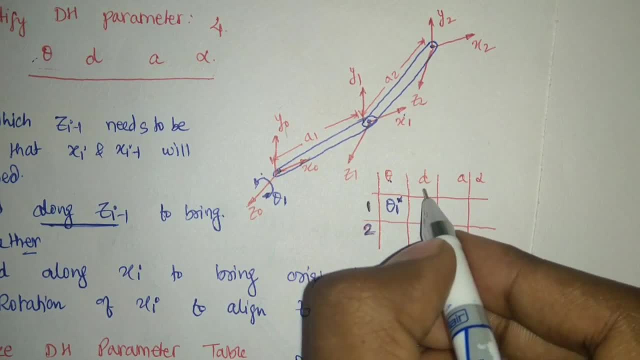 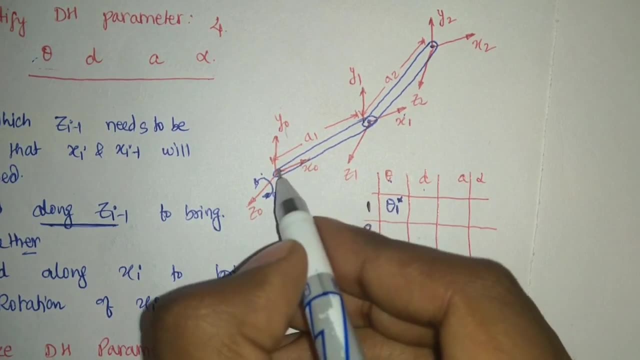 write them directly. Okay, So theta1 here now d, is the distance along zi minus 1, so along z0, how much distance I need to move so that these two origins will get aligned with each other? okay, so z0 and 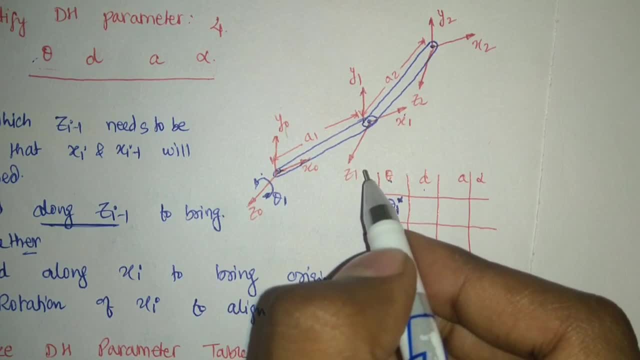 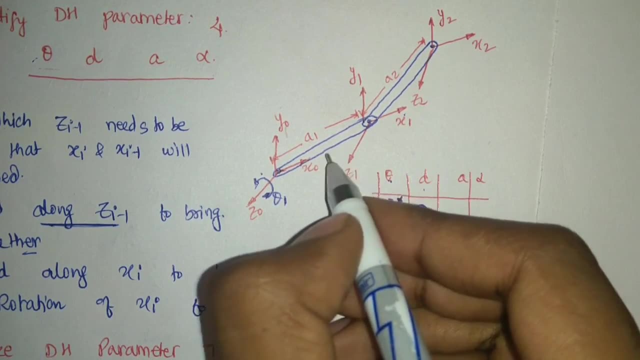 z1 are both parallel to each other. there is no distance that I can travel to bring them closer. okay, so that becomes 0 over here Now. next one is a. that is the distance that I need to travel along x1,. okay, along x1. 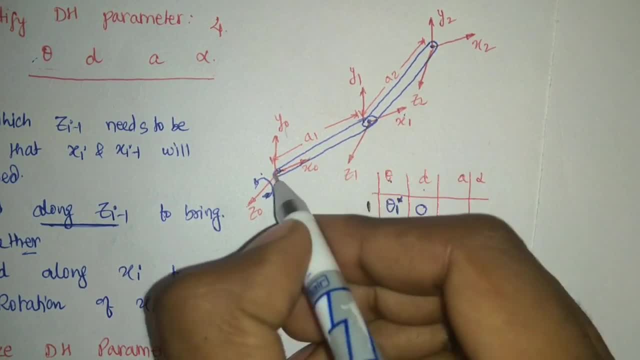 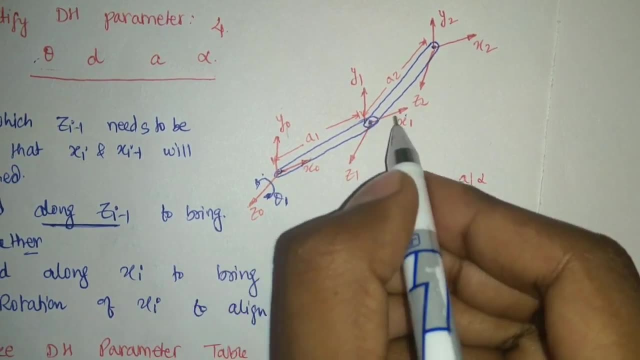 so that now x1 and this, This origin and this origin will come closer or at the same point. okay, so how much is that distance? It needs to travel a1 distance. okay, along x1, I will need to travel a1 and then only. 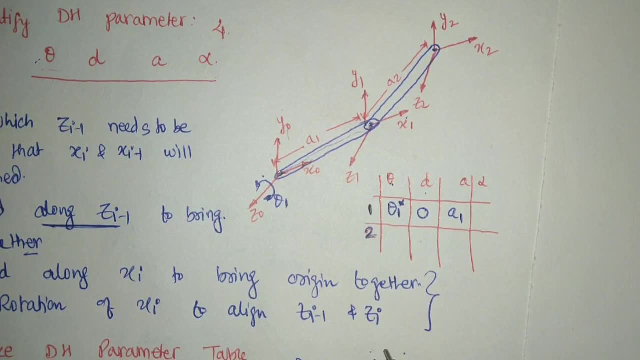 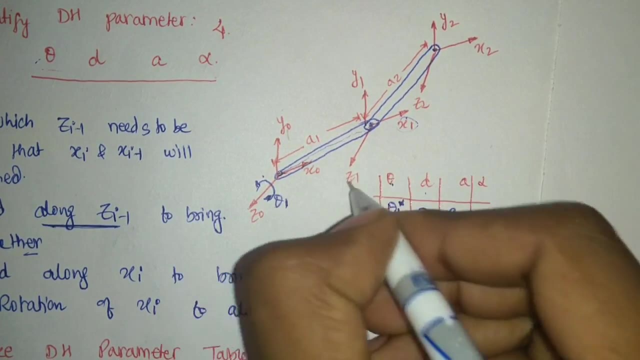 they will get aligned. the two origins will get aligned. Now, alpha is the angle with which I need to rotate x1, so that z will get along with each other or z will get parallel to each other. so they are already parallel to each. 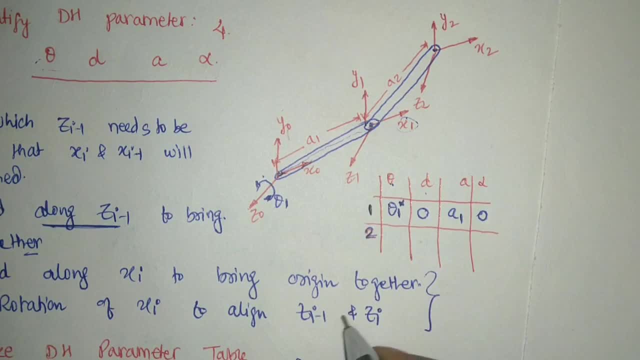 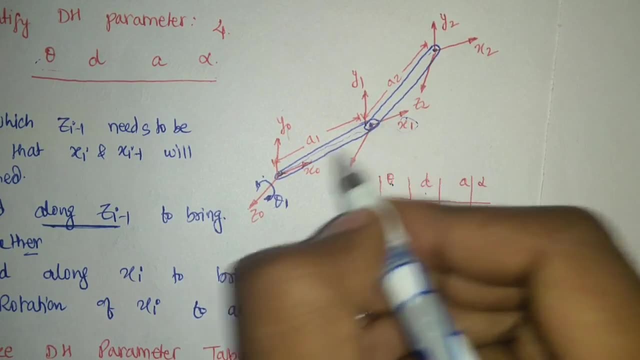 other, so I need not rotate my x. Similarly, when I talk about second row here, then between this and this frame. so again this is the same case, only so z1 needs to be rotated with an angle, theta2, which is a. 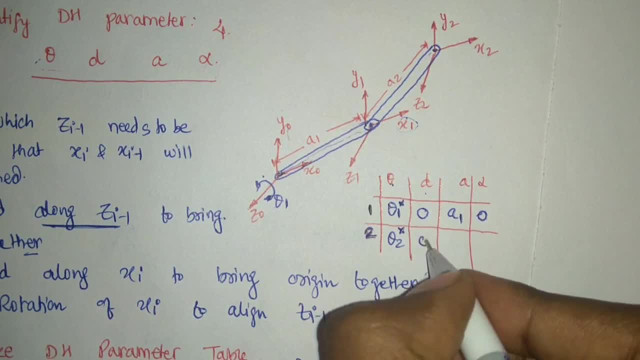 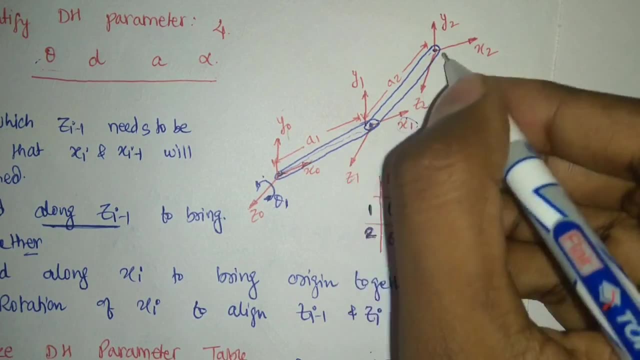 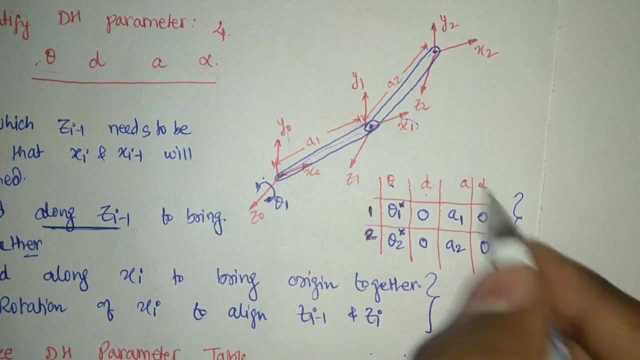 joint parameter, so I will put a star over there. okay, there is no distance that I can travel along z1, then a2 will come here, because along x2 I will need to travel this two length and then alpha will be 0,. okay, so that is how we make the dh parameter table. this is: 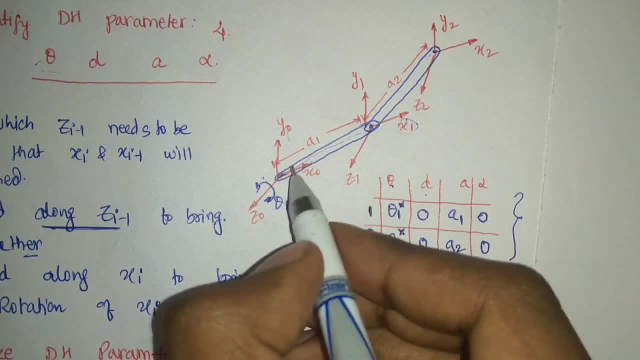 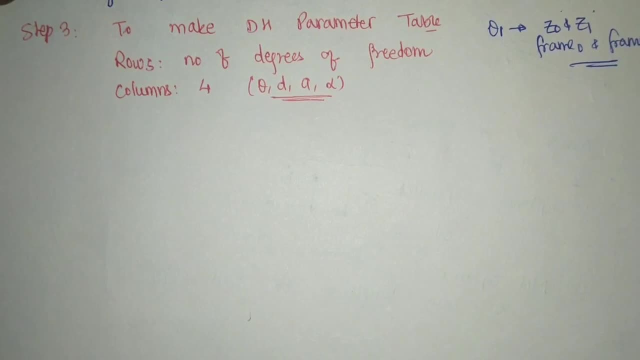 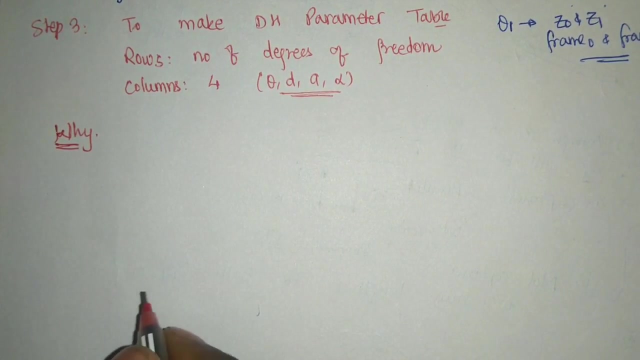 for a 2 degree of freedom. Now we will understand the significance of doing this thing. okay. why exactly are we doing it this way? now, let us understand that significance first. okay, now the question that can be raised here is: why exactly are we having these four parameters and how exactly? 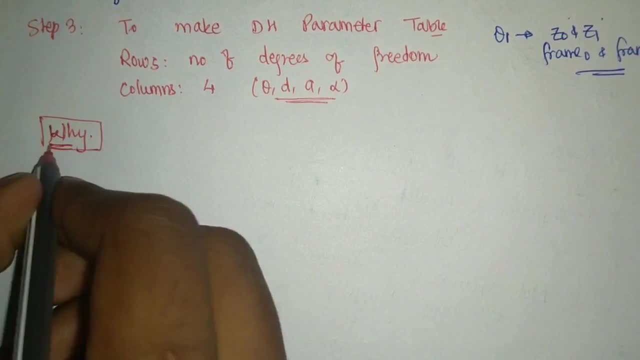 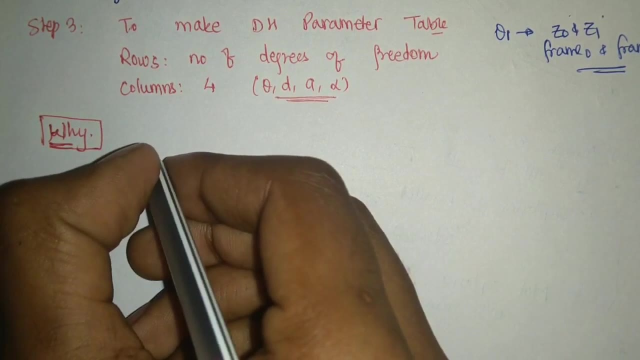 will that help us? okay, because you need to understand this, also in order to be able to grasp the concept better. okay, so why exactly we are doing it? so here we are, basically having concept of moving frames. okay, we are moving the frames. we are moving the frames. 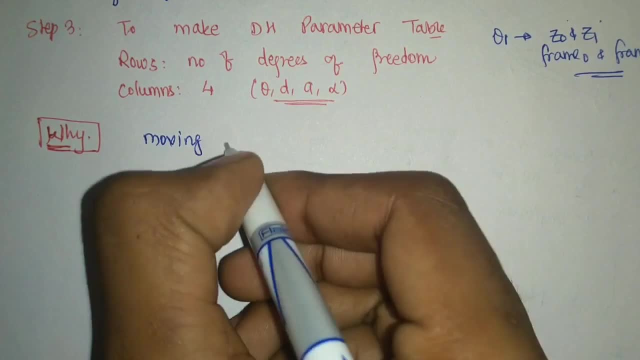 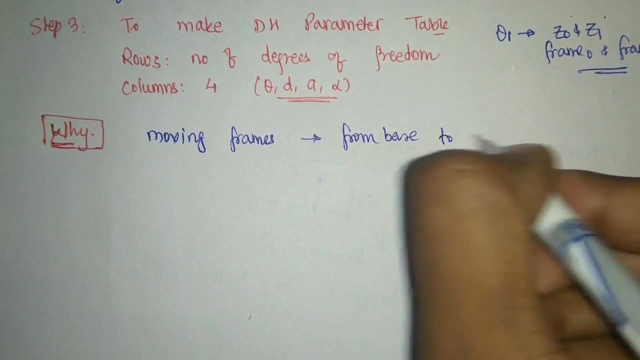 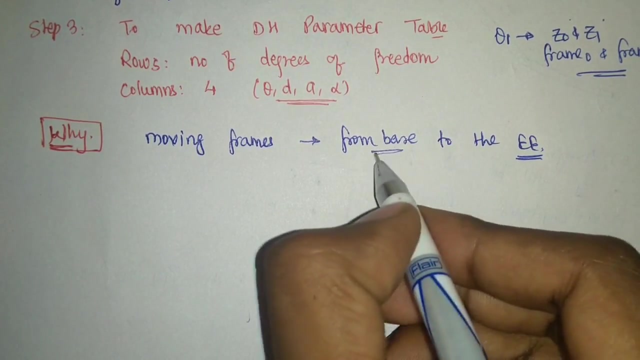 in order to align them together. okay, so we are having the concept of moving frames and we are going from the base. okay, we are going from base to the end effector because we need to know the actual location and the orientation of the end effector. so, from going, 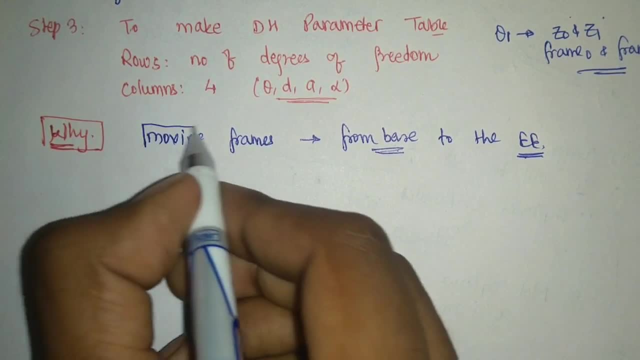 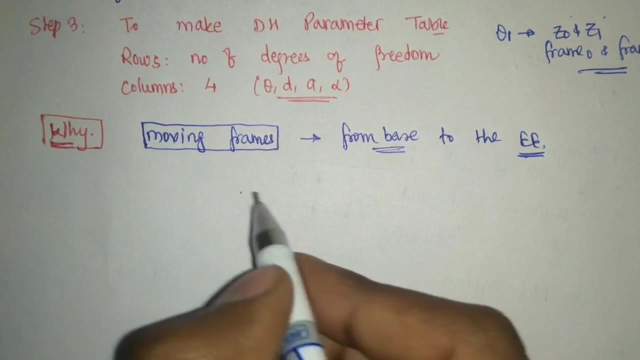 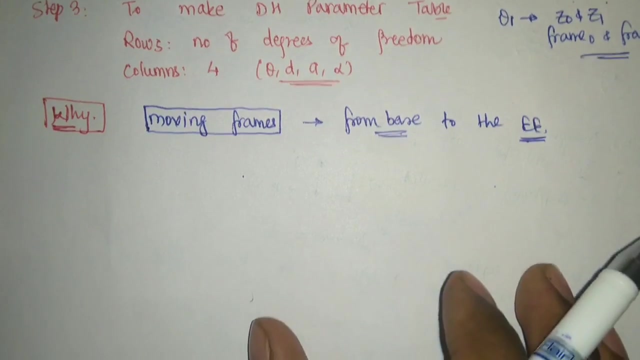 going from base to the end effector. we are using the help of moving frames. okay, and these moving frames are what we assign to each of the joint, and then, from the base, we move right up to the end effector. That is why we are having this all 1 to 2 to 3 to 4 and so on. okay, now how exactly? 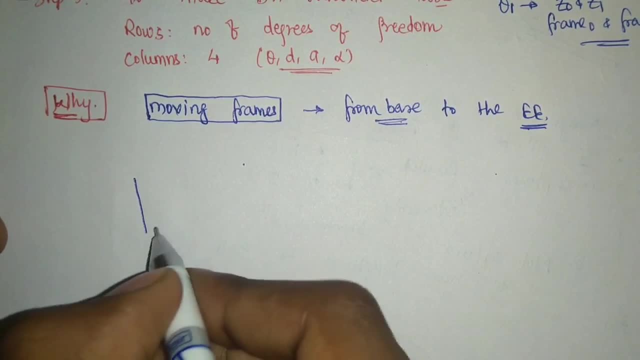 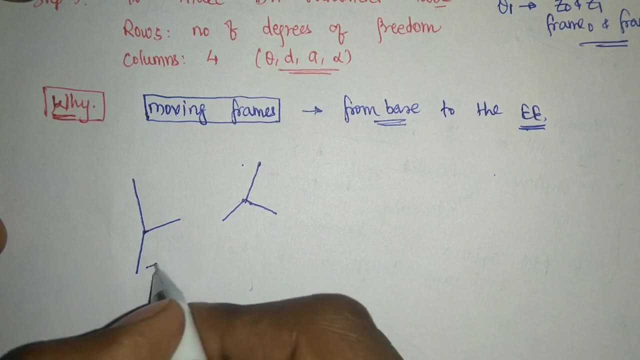 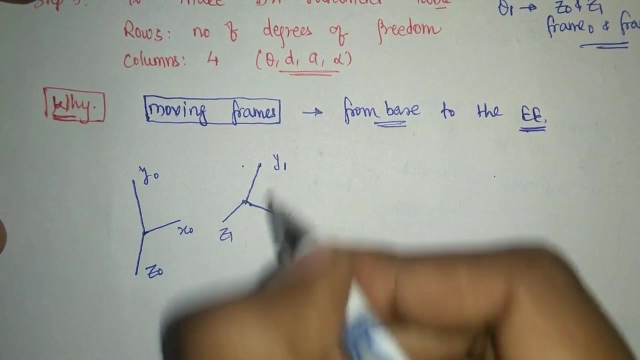 that is helping us. so let us say I was having these any arbitrary two frames over here that I had initially given, let us say Z0, Z1, X0, X1 or whatever, why it does not even matter to us because we do not care about that. so the first thing that I am going to do here: 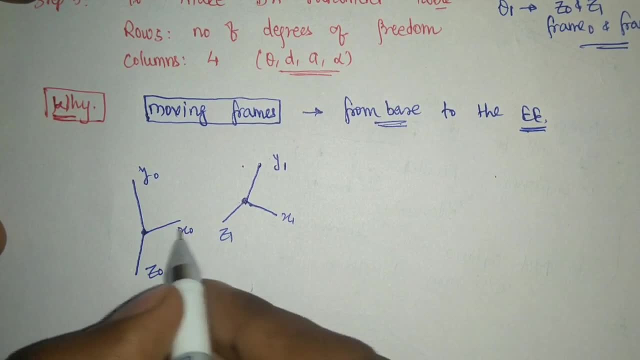 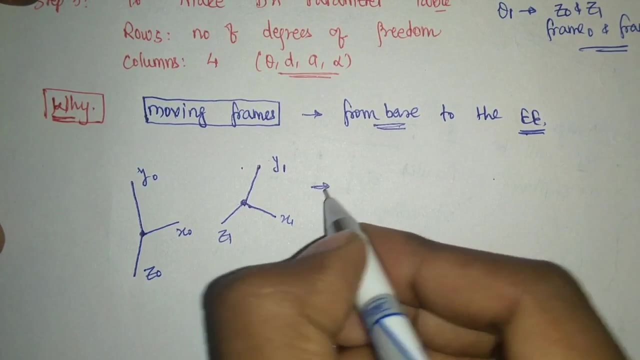 is, I am going to align, Okay, These X's together. okay, so I will simply rotate my Z so that I can align X together. so that will give me, with the help of theta- I will be basically making it like this- this: 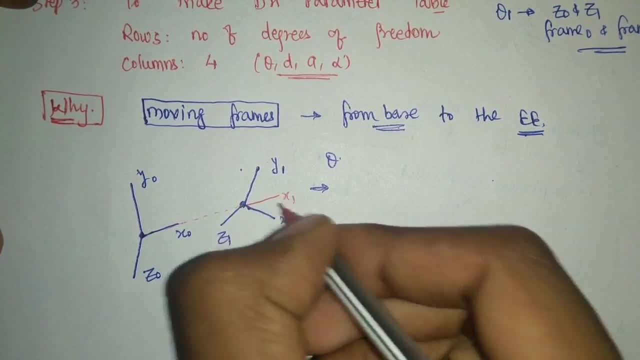 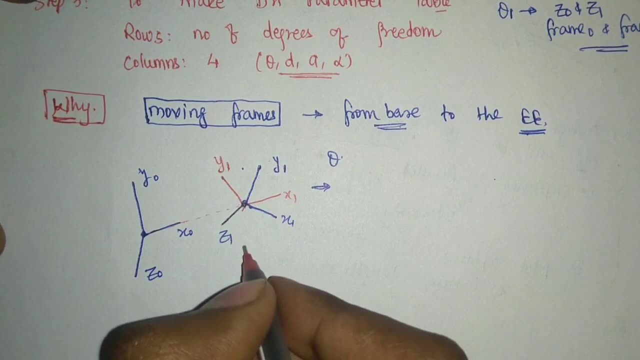 is my X0 and X1 will come here. okay, so basically I am rotating it right. Z will remain where it is, Y1, because I am rotating about at Z1 anyway. okay, so that gives me X1,, Y1, Z1. 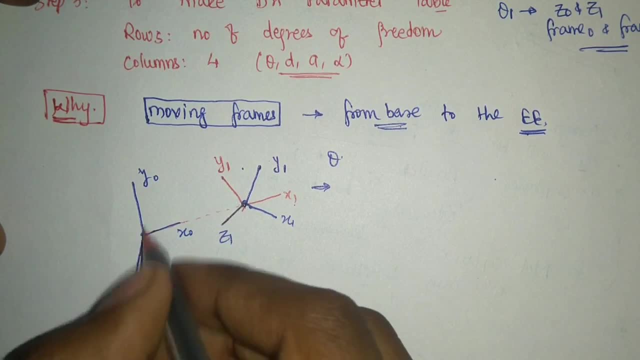 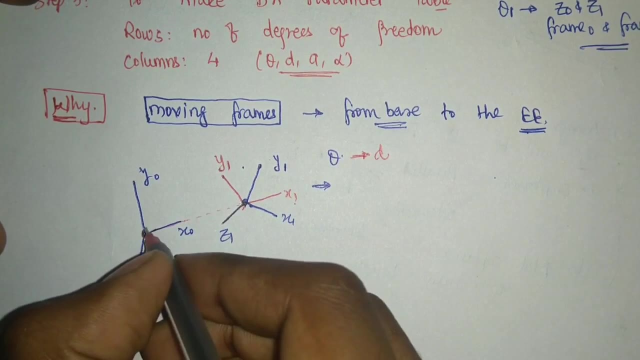 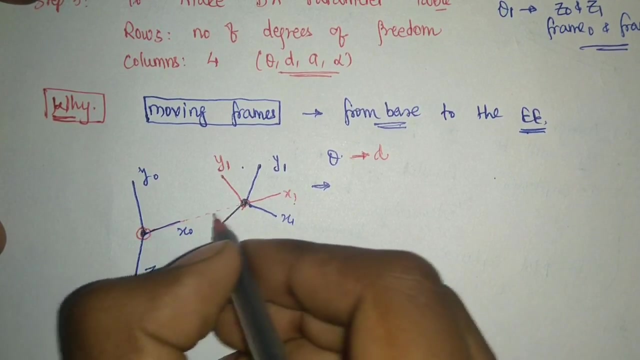 and I have done it right. second thing is: I will move it along Z axis. so if whatever possibility is there, then I will move it along Z axis, otherwise not, so that I can bring these two along same line. okay, and what the same line would be along X axis they. 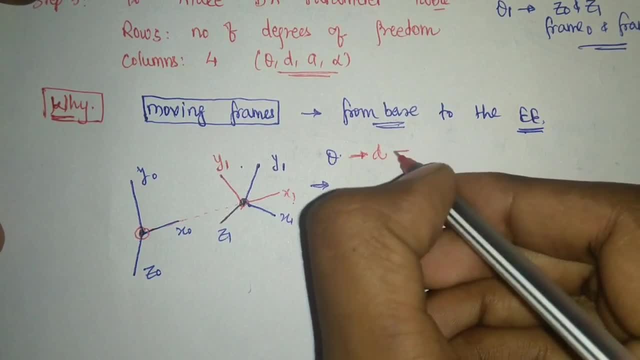 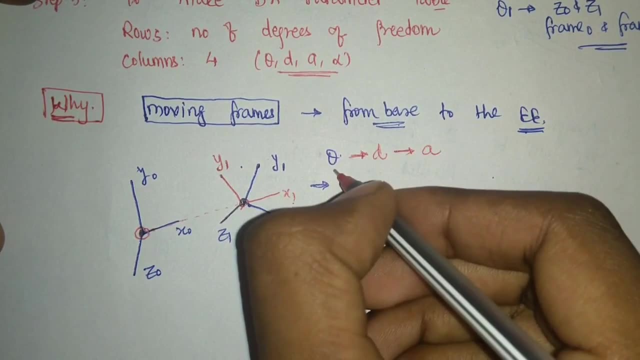 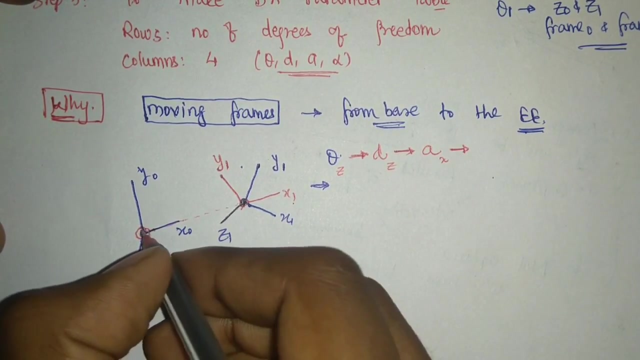 will come along X axis together. okay, so that is D. then, since the X axis has now aligned together, now I will move it along X axis. so now I will have this A, so theta about Z, Okay. Okay, Then A about X I am having here. then next step will be when I have moved this frame. 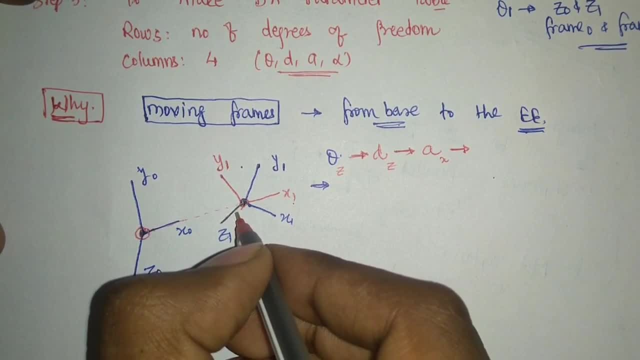 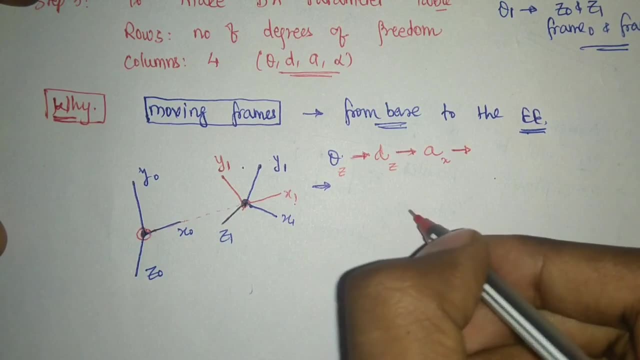 to here or this frame to here. it basically doesn't make any difference, right? so I am basically moving this frame to this location, so they will come together, right? so what I will be having after this is I will make these two frames here. this is my initial. 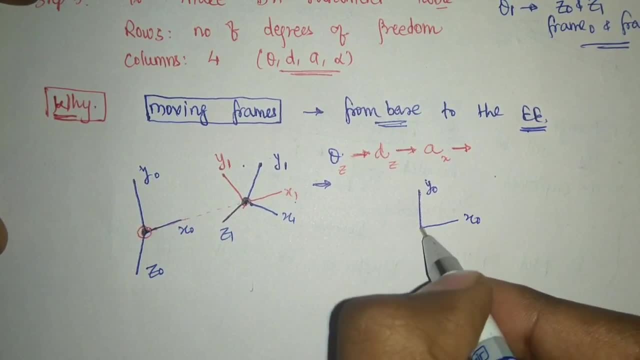 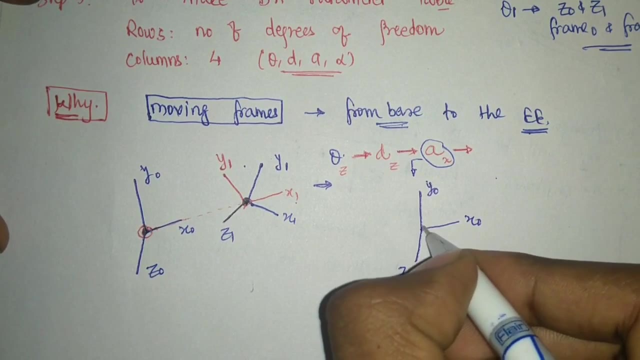 frame Y0, X0 and this was my Z0, now, after A, I am moving this frame to here. so I am moving AX and after having moved along X1, what I will be having- that my axes are aligned. 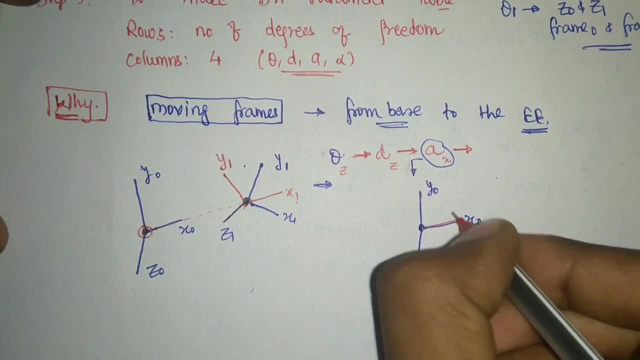 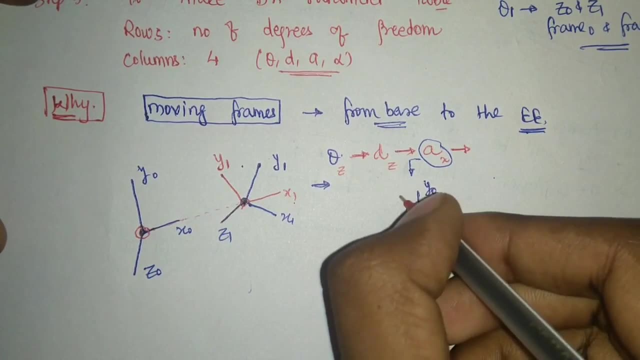 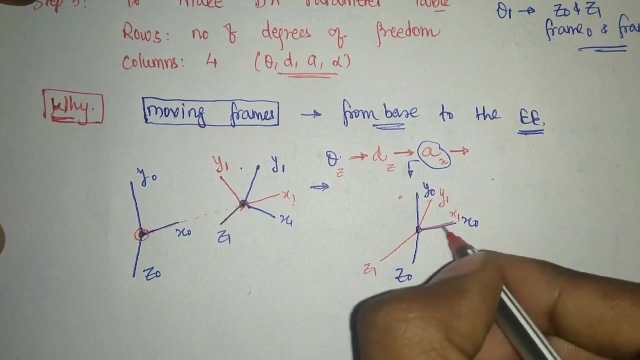 together. now my X0 and X1 are aligned together, but my Z1 and all those things are having some issue. that is Z1, and somewhere I am having my this Y1 also. okay, Y1,. now what I will do? I will rotate it along X axis so that Z can come together. okay, so then? 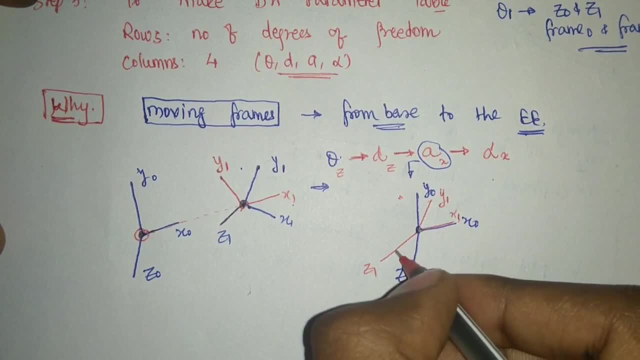 I will be having alpha, So alpha along X axis in order to make the Z come together. now Z will come together, so whole frame will get aligned together. both of these frames will get aligned together, and that is what we have wanted. that is how we can calculate it right now. this sequence: 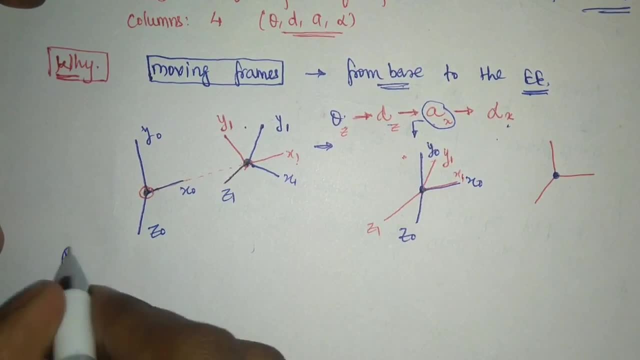 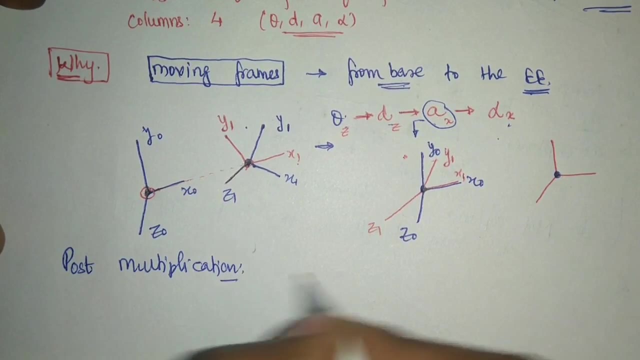 has to be followed here, and we are moving the frame means it is a case of post multiplication, right, we are having a case here of post multiplication. so in order to calculate the individual transformation matrix- okay, Transformation matrix- each individual transformation matrix is consisting of these four operations. 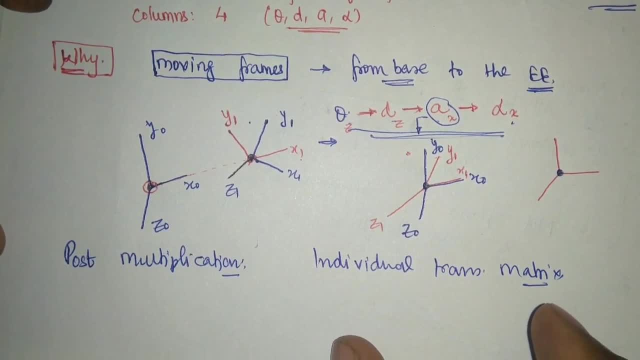 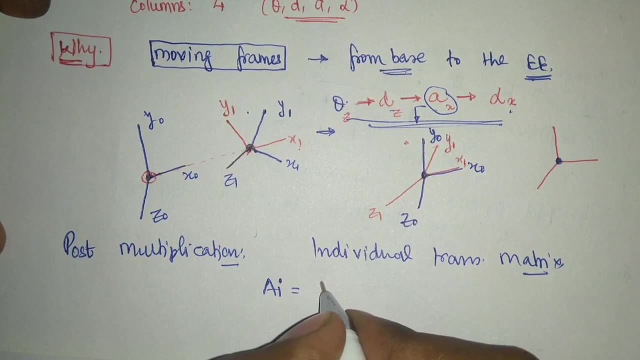 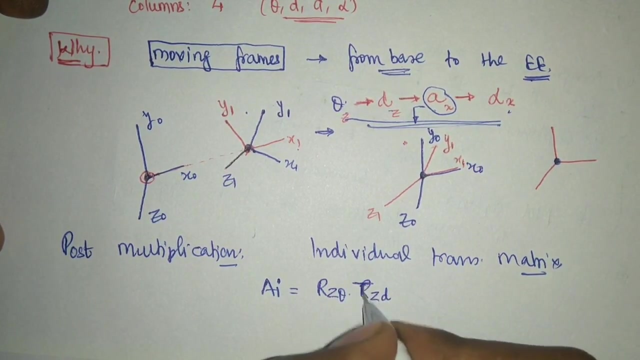 whatever is 0, we will put that 0 anyways, but we will be having these four operations. so any matrix, Ai will be Ai represent for this transformation matrix here, RZ, theta and post multiplication. we are doing then RZD, sorry translation along ZD, then translation. 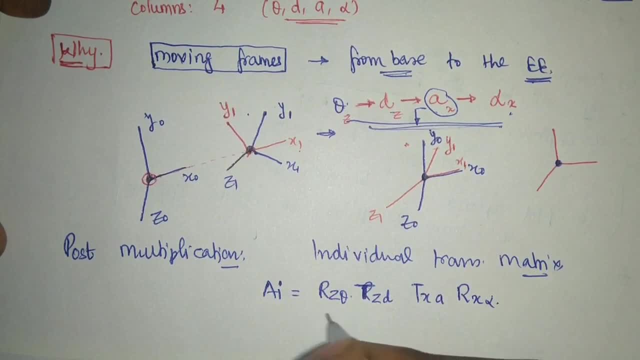 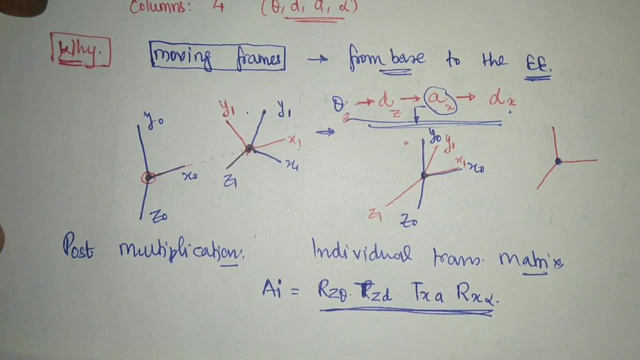 along XA and then rotation along X, alpha. Okay, So we will calculate this individual matrix here first, and then we will move towards the overall transformation matrix. okay, This I am telling you so that in case you do not remember Ai formula, then you can calculate. 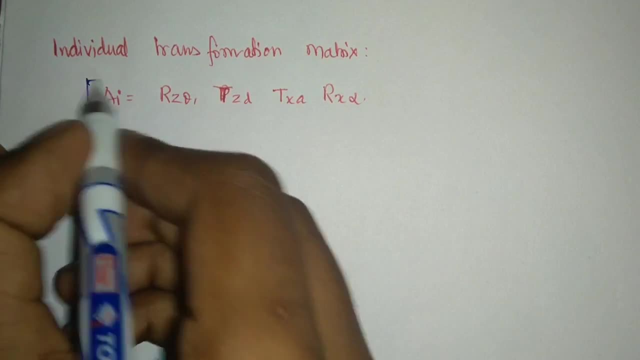 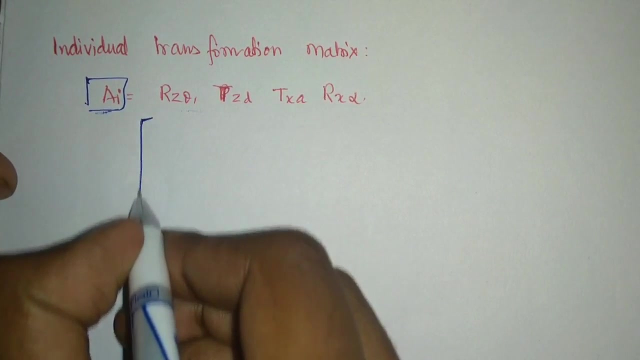 it on your own in the exam, right? because anyways you will be needing to calculate AIs and overall matrix, and for that you will either carry out the transformation or remember the formula directly. that is up to you Now. RZ theta is nothing, but it will be C theta 1 minus sine theta right or C theta. 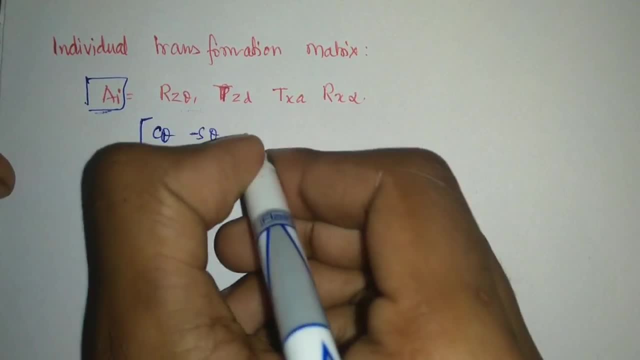 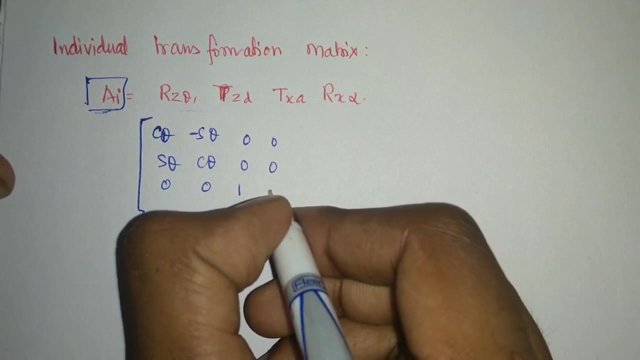 minus sine theta right. So RZ theta is nothing, but it will be C theta 1 minus sine theta right, or C theta 1 minus sine theta right. So RZ theta minus sine theta, then 0, 0, sine theta, C theta 0, 0,, 0, 0, 1, 0, and 0, 0, 0, 1,. 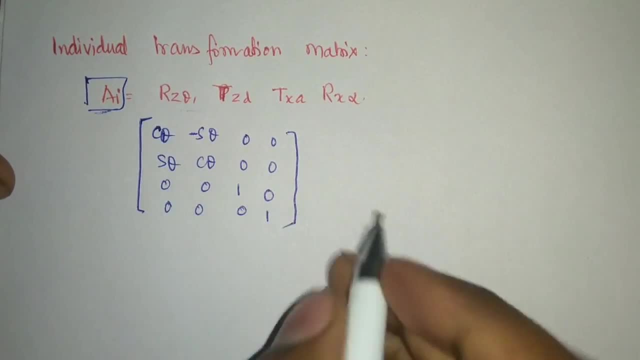 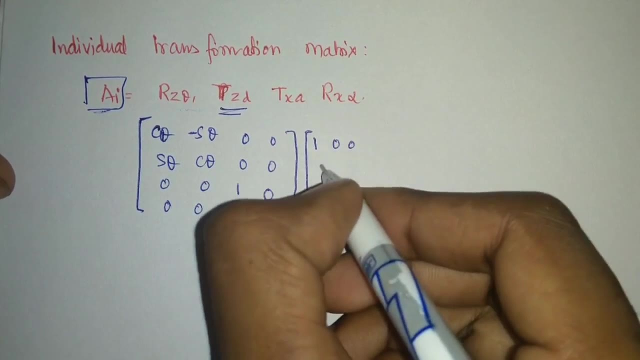 right, That is the 4 by 4 matrix for RZ theta, right. Similarly, I will be having a 4 by 4 matrix of TZD, also right, and it will be 1, 0, 0, 0, 1, 0, 0, 0, 0, 0, 1, triple 0, and then the transformation part, that is 0, 0 and then 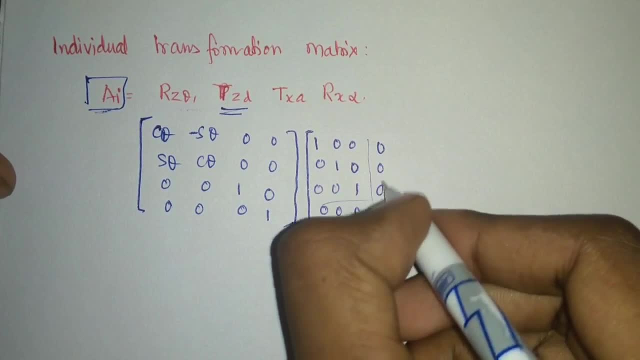 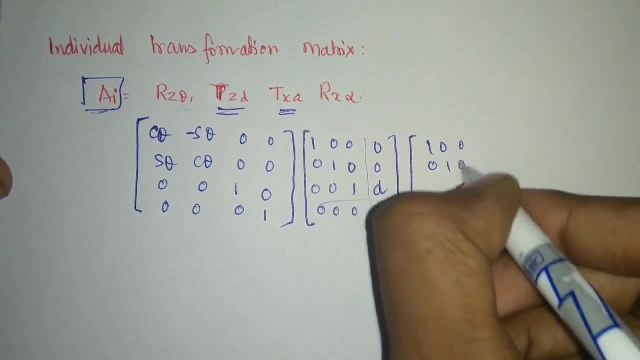 piece 1.. Okay, So RZ theta will be 4 by 4. and I am having transformation along Z and B at the same time and then transformation along X, so that will become 0 0 0, 1, 0 0, 0, 1, and here it will become A 0 0, triple 0, 1. 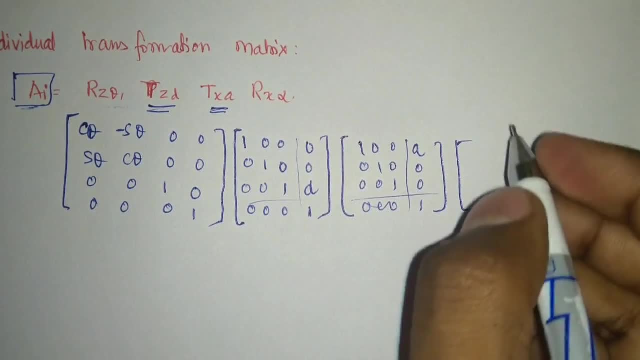 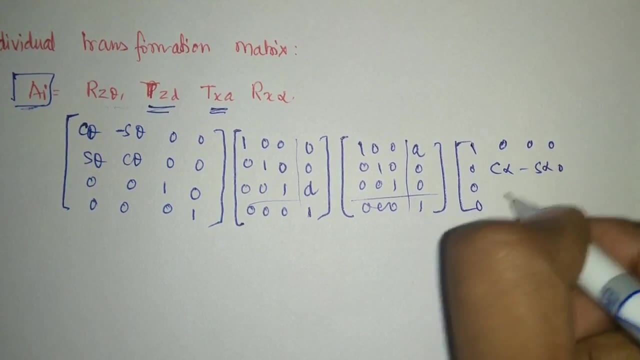 right. and then my, finally, rotation along X axis. and rotation along X axis also, I know the formula or I know the matrix already very well. right, C alpha minus S alpha 0, 0, 0. sorry, S alpha C alpha 0, 0, 0, 1. now that I can now multiply with each other in order, 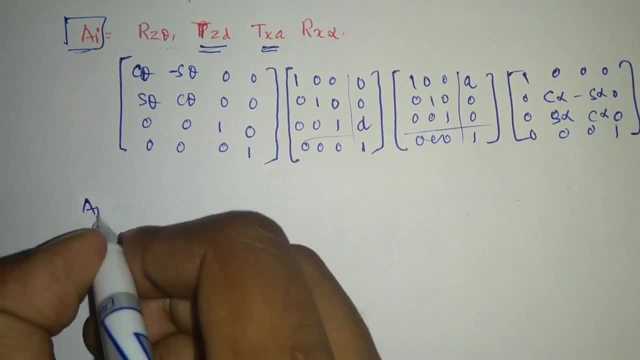 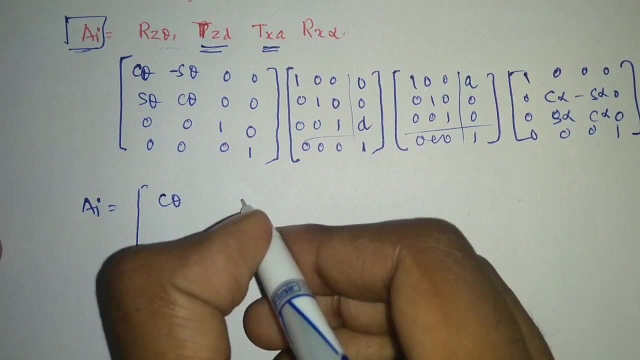 to calculate the final A I matrix. okay, and A I will come up to be equal to. that is the final expression that either you remember this expression or you can calculate in the exam using these four transformation, in case you don't remember it. okay, this is the main. 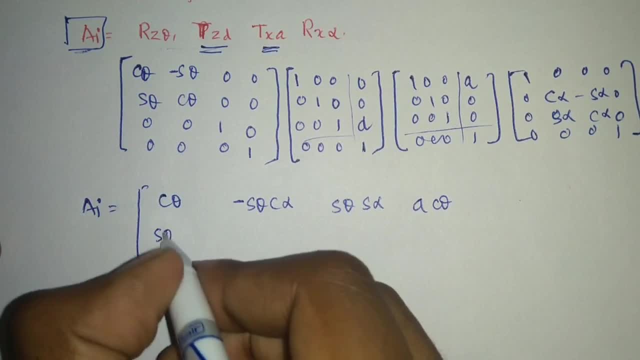 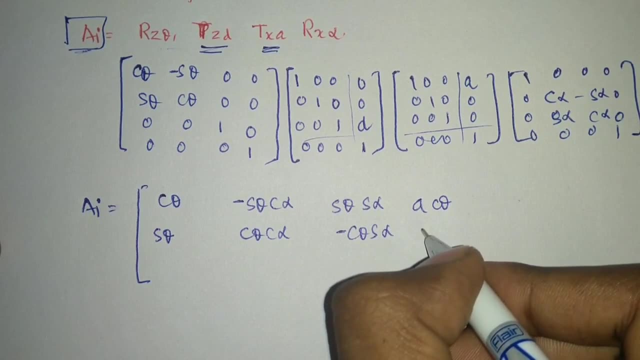 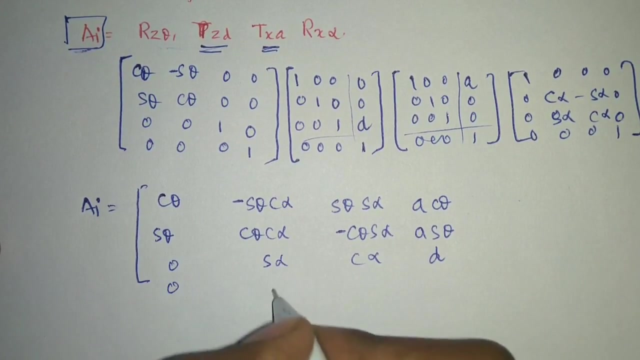 stripe question only In prelims. They can only ask the steps or the conditions for different different steps that we are following over here. right, they will not ask the formula anyways, but let's have it for the main point of view. 0 0, 0, 1. now that is my A matrix. I can directly use this matrix. 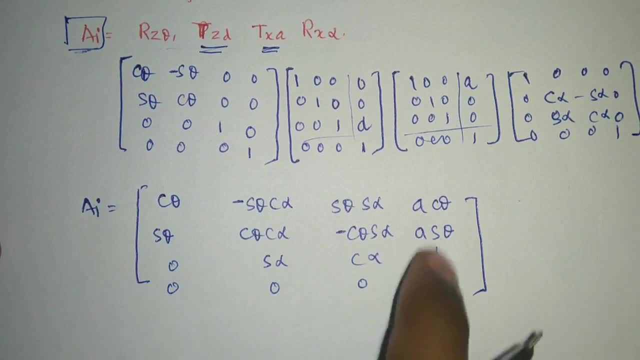 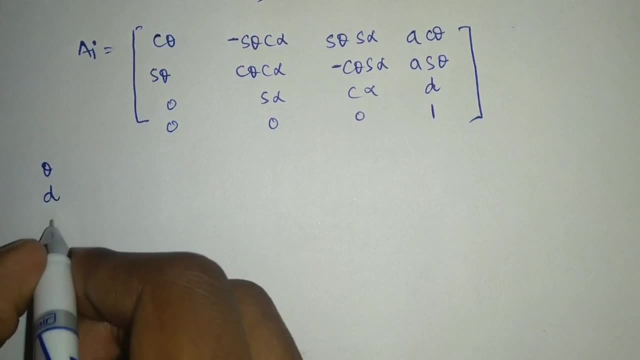 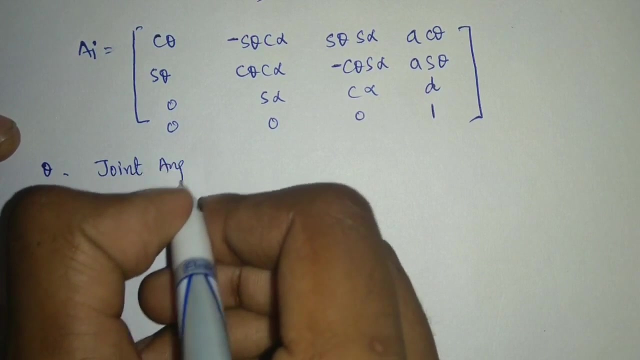 once I know my parameters theta, alpha, A and D. okay, now, usually you will also see this convention that This parameters theta, D, A and alpha are known as or are called with different names also okay, so A is basically okay. theta is basically joint angle. okay, whatever joint angle we are. 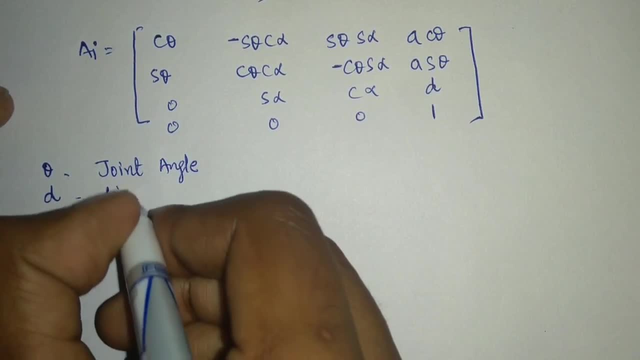 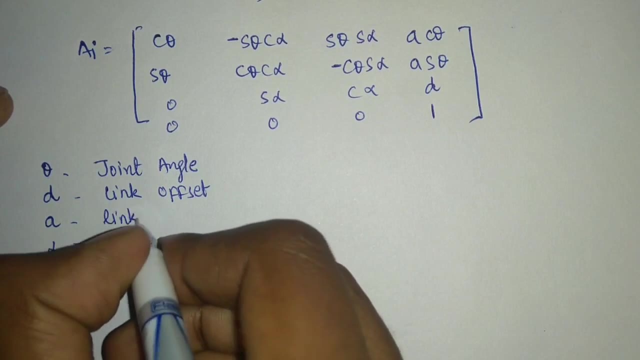 having over there. then our D is link offset. it is known with the link offset, okay. then our A is link twist: 0.1.. 0.2. 0.3. 0.4. 0.5. 0.6.. 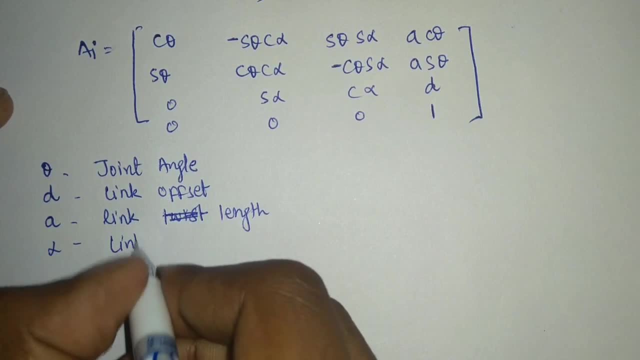 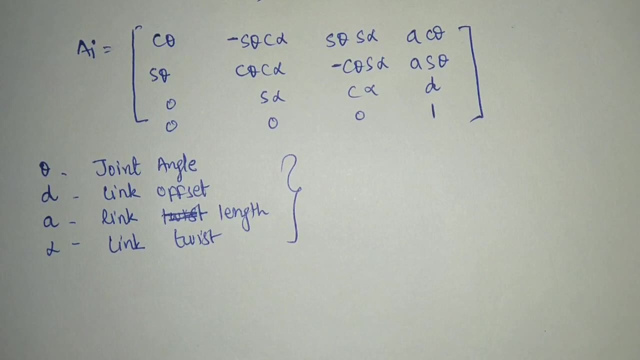 0.7. 0.8. 0.9.. 0.10. 0.11. 0.12. 0.13. 0.14. 0.15. 0.16. 0.17.. 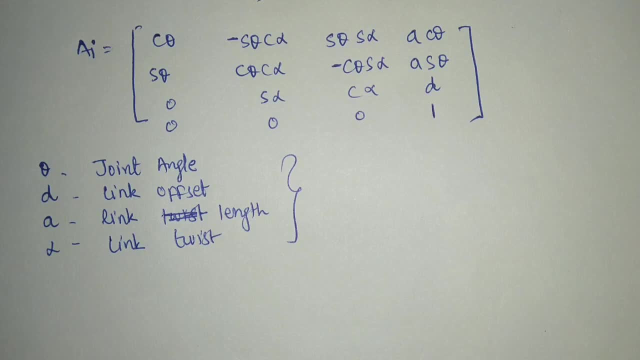 0.18.. 0.19.. 0.21., 0.22.. 0.23. 0.24.. 0.25. 0.26. 0.26. 0.27. 0.28.. 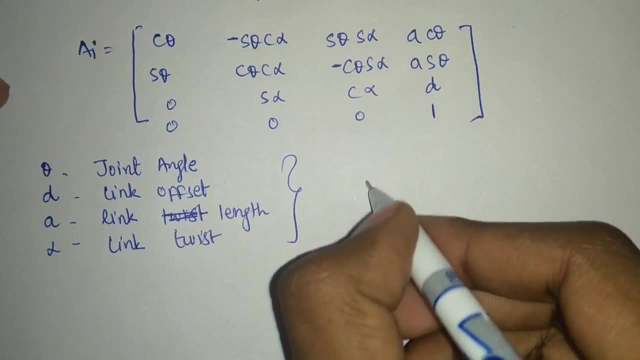 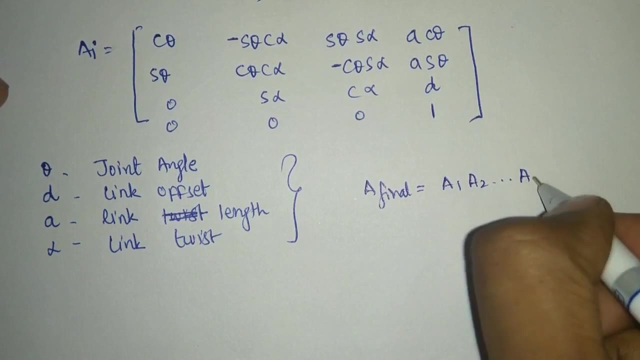 0.29. 0.30. 0.31. 0.32. 0.33. 0.32. 0.34. 0.35. 0.35. 0.36. 0.37.. 0.38.. 0.39.. 0.41.. 0.45.. 0.46.. 0.49.. 0.51.. 0. 0ENo 0.56.. 0. Sei. 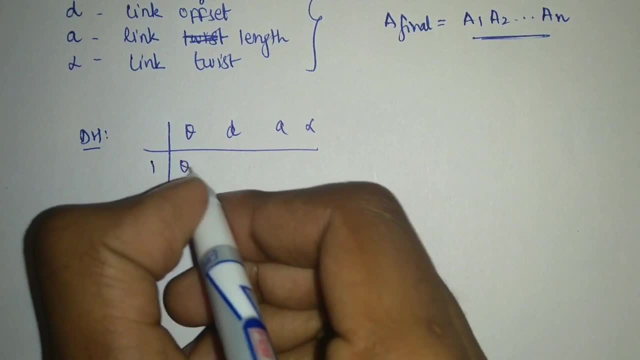 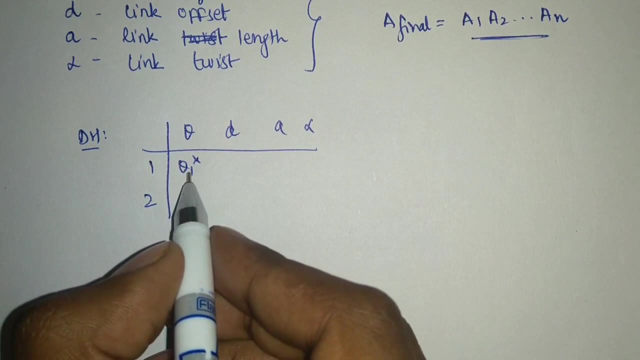 0.56.. 0.57.. 0.58. 0.59. 0.52.. 0.53. 0.55. 0.うわ. joint parameter: if it is a rotatory joint, then we will put a star, and if it is a sliding. 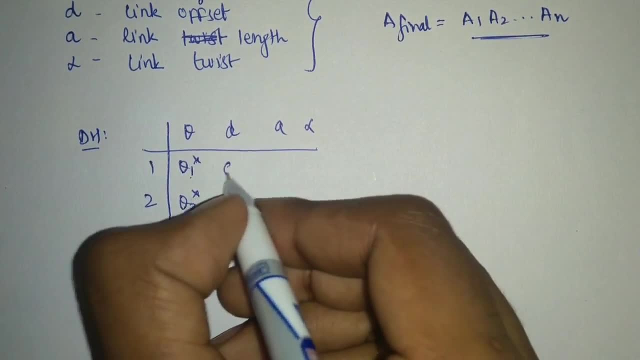 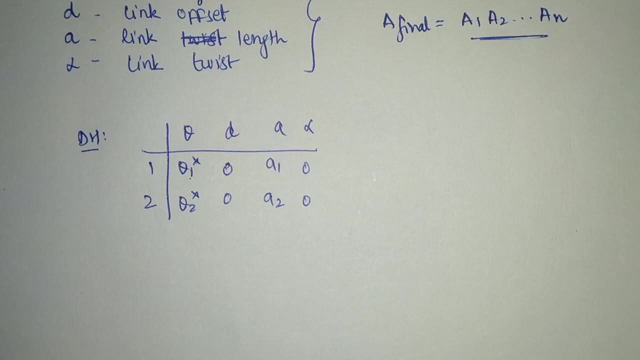 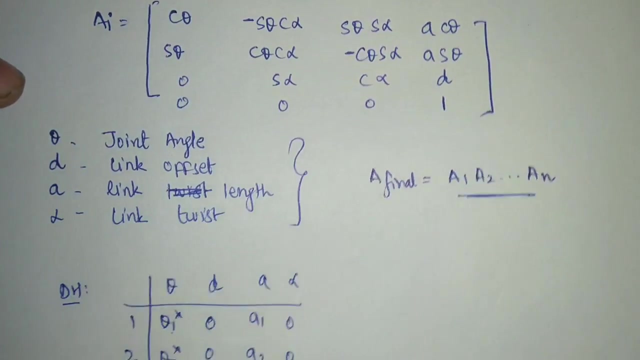 joint. then we will say d star. that way, d was 0,, a was a1 and a2 and alpha was also 0. so this was the matrix that we had calculated earlier. now apply this matrix. with the help of this a, we will calculate the individual and the overall transformation matrices. so 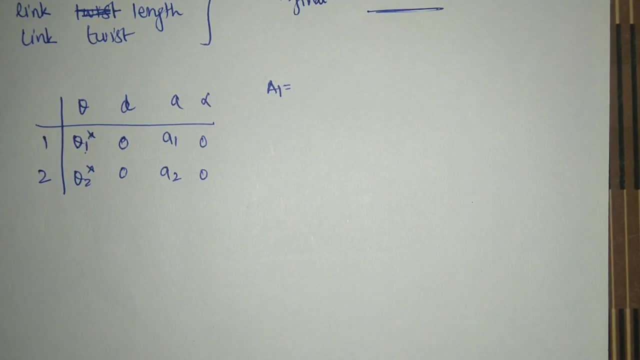 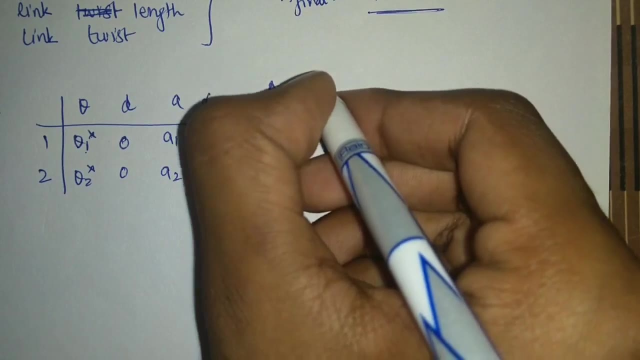 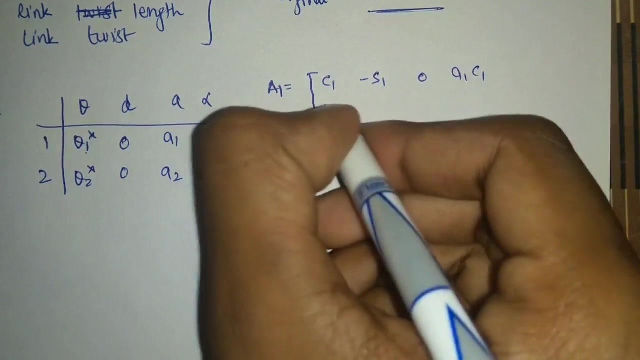 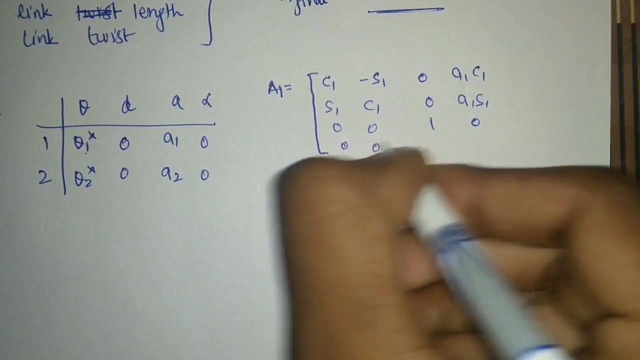 a1 will become. how much will a1 become? I am going to apply all these values here, so a1 will be. basically it will become c1 minus s1, 0, a1- c1, s1- c1, 0, a1- s1, 00100001. 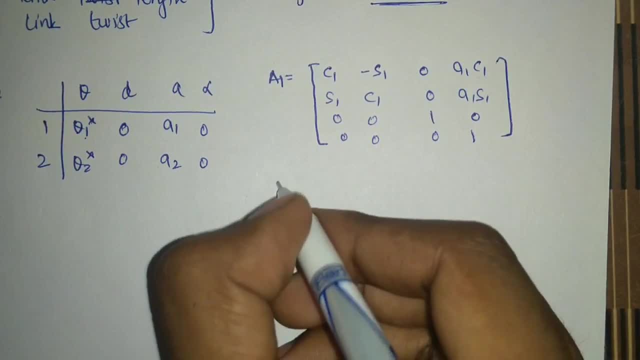 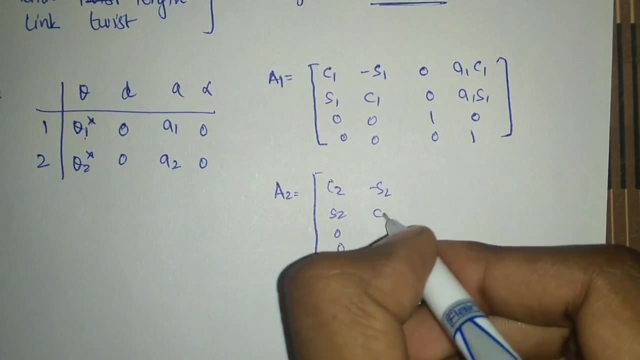 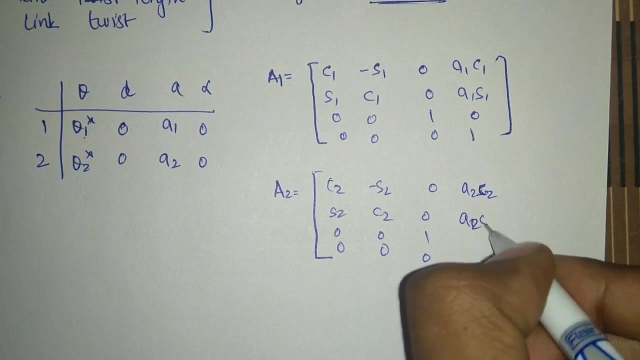 you can calculate it. we will simply put the values in the above matrix that we have now, just calculate it and you will get it similarly: c2, s2, 00, minus s2, c2, 00, 0, a2, c2, a2,. 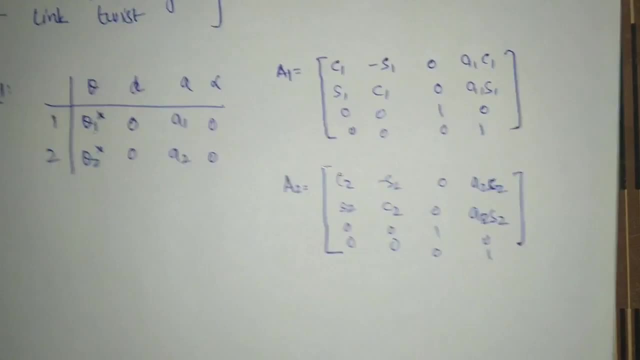 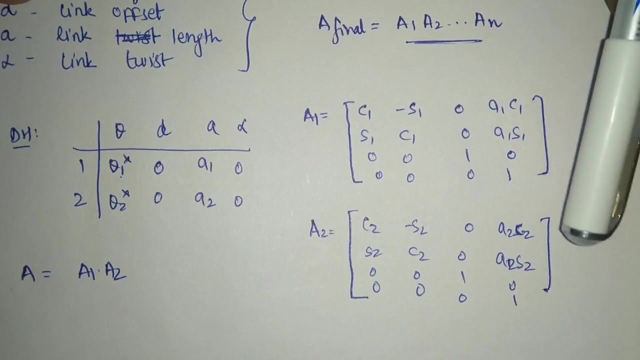 s2, 0.. so we have calculated both the matrices in order to calculate the overall matrix. a is equal to a1 multiplied by a2.. now let's do the multiplication so that we can calculate or we can get the final matrix here. 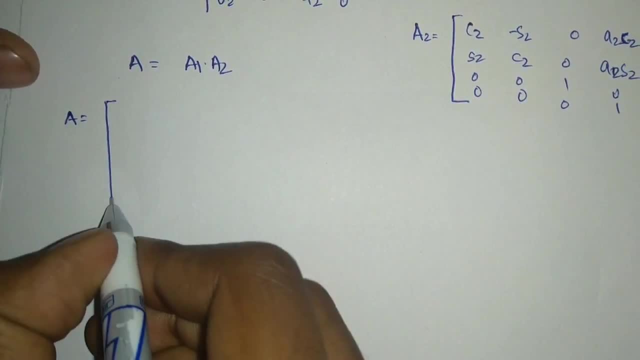 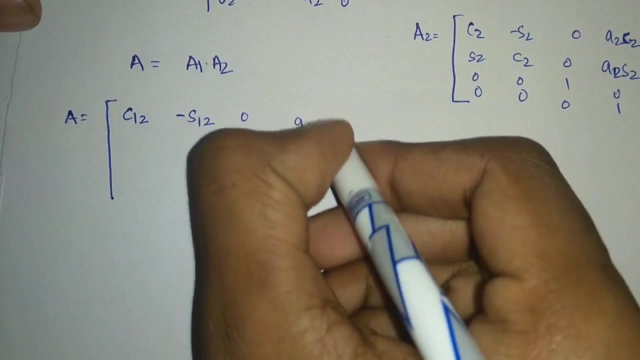 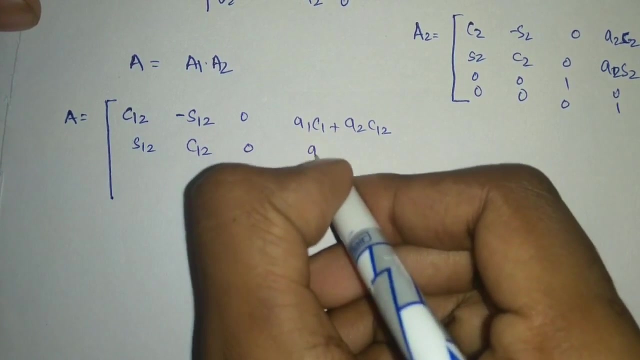 a will be equal to this. multiplied by this, and if I calculate the multiplication here, that will come out to be c12 minus s12, 0, a1, c1 plus a2- c12, then s12- c12, 0, a1- s1. 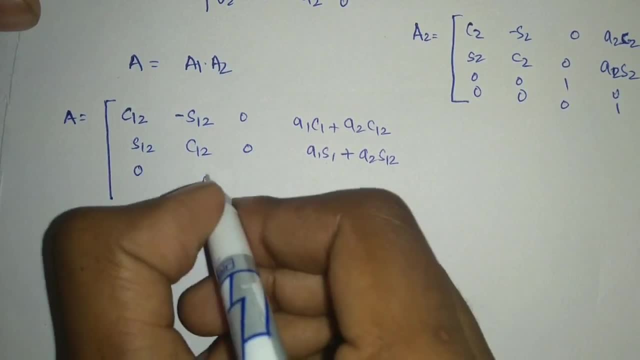 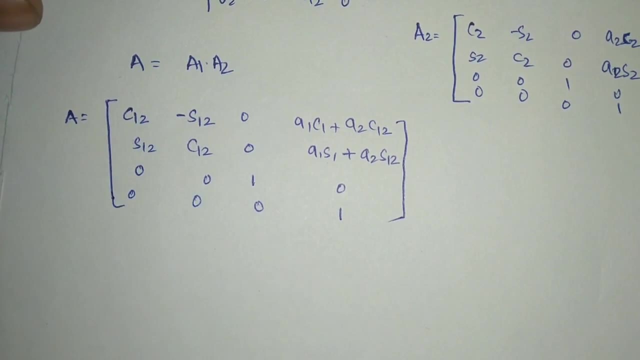 plus a2, s12, and then 00,, 10,, 00.. okay, that is what we have calculated. so now we will have got an overall transformation matrix for the two degree of freedom system that we had started with. now, in this two degree of freedom system or whatever final matrix. 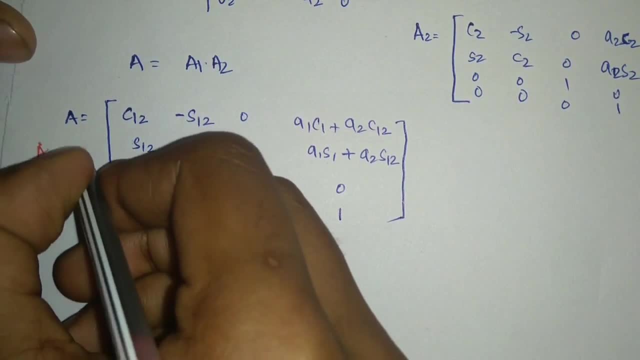 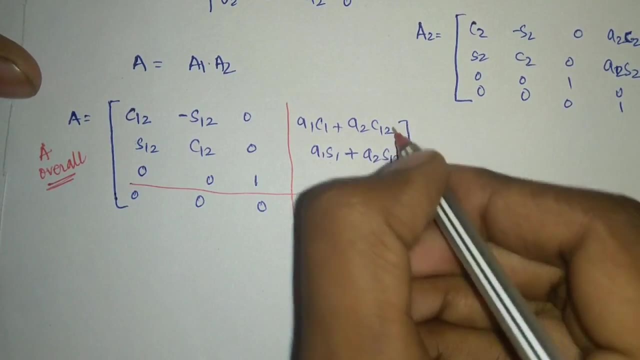 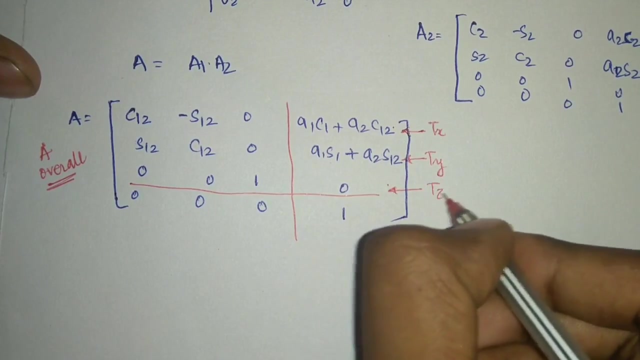 that we get a over right. so in the overall matrix, in order to calculate the tool position: okay, so tool position will be given by these three points here. so this will be the tool's x position, tool's y position and this will be tool's z position. okay, and this will be. 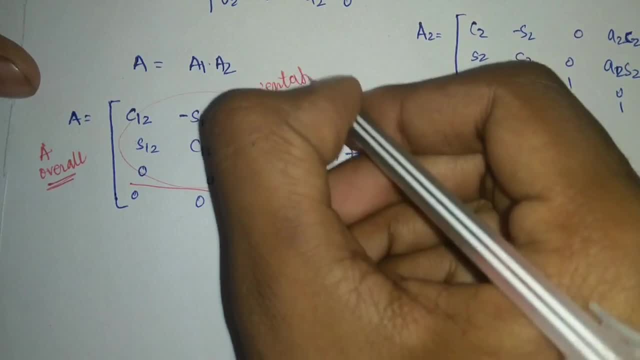 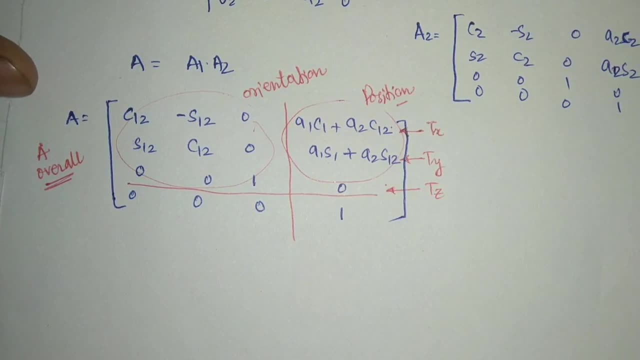 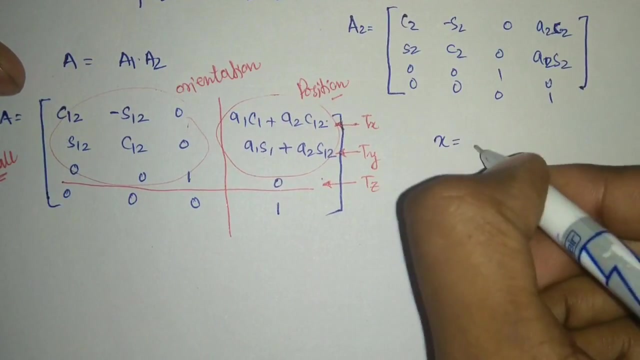 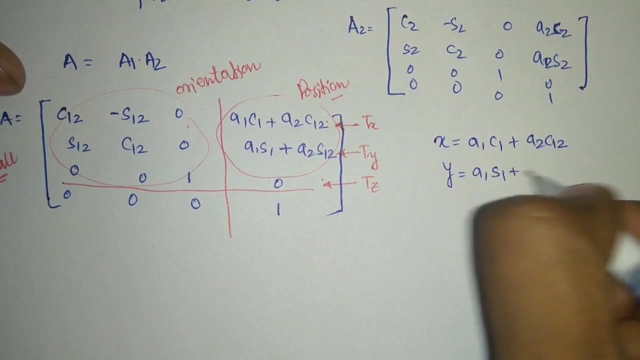 orientation matrix. So this is the orientation and this is the position of any tool. Usually we are asked the position only. So, finally, what I can say? that my tool or my end effector is going to have x coordinate as a1, c1 plus a2, c1, 2 and y coordinate as a1, s1 plus a2. 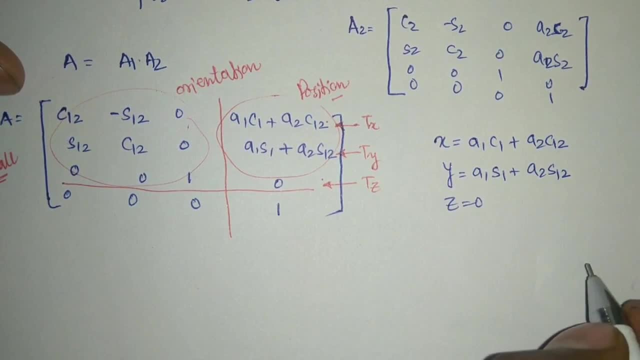 s1, 2 and z coordinate as 0, because we are not bothered about z coordinate here. Now you can match these values with our graphical analysis also or our geometrical analysis. We have got same values there also in our direct kinematics, So that is how we can calculate. 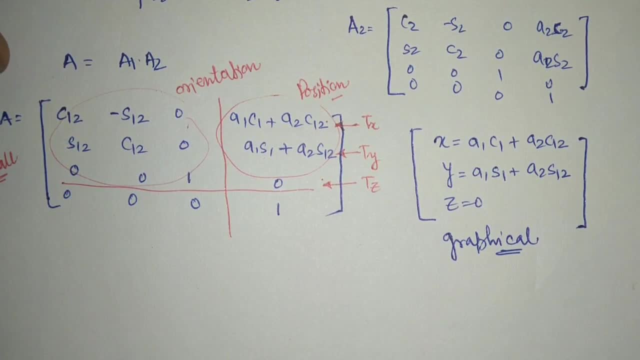 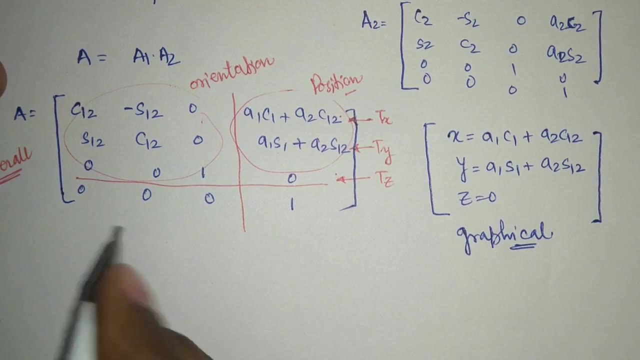 the values over here. Now the next part of the question. the question that we saw in the beginning of this video is regarding if a1 is given as 15, a2 is given as 10, theta 1 is given as 45 degrees. 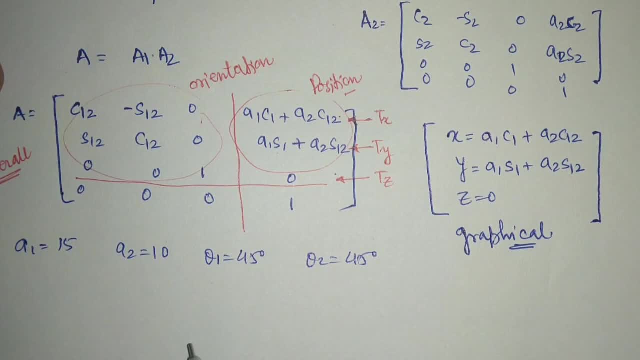 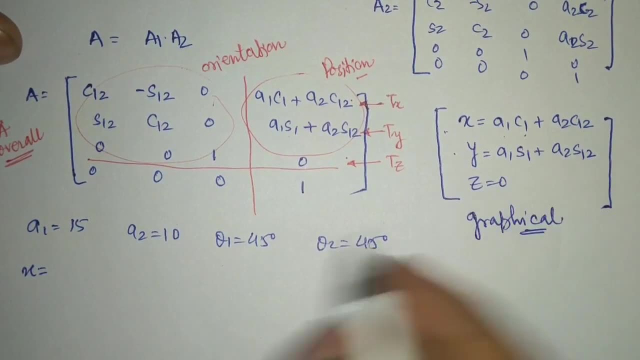 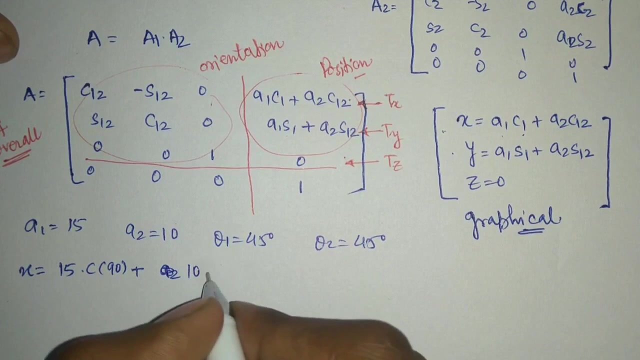 Then we need to calculate the position as well as the orientation. So position is x, y and z. So x is equal to a1. c1 means 15 cos of 90 degrees plus a2, a2 is 10 into cos of. 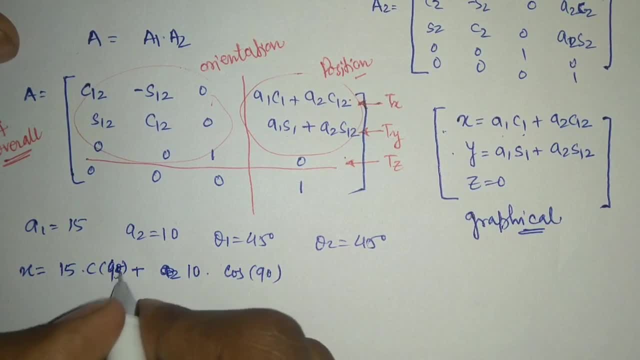 90. This will be c1 plus c2, this is 45 degrees Cos of 45 degrees, and that will be. that will become how much: 15. 15. 15., 15., 15. 15.. 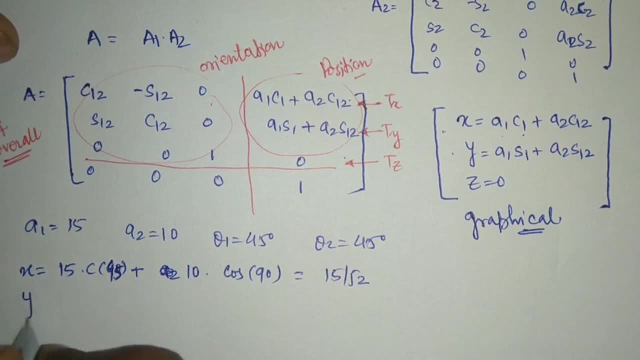 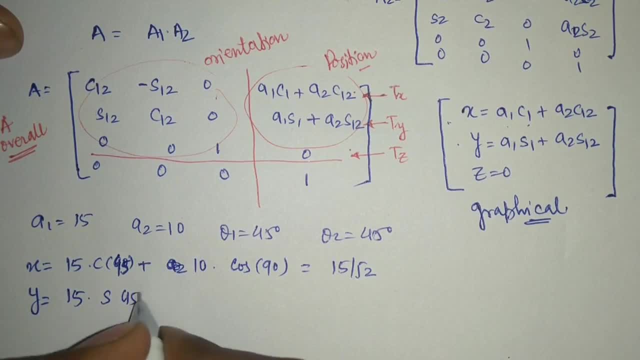 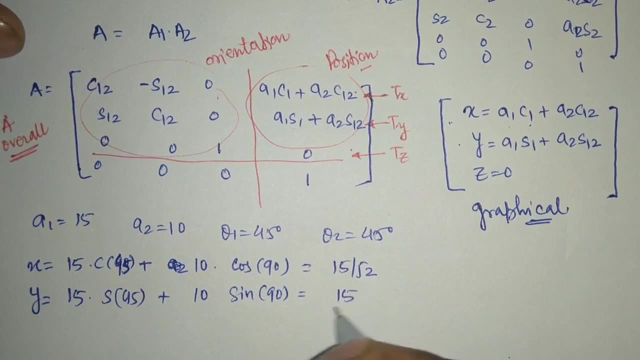 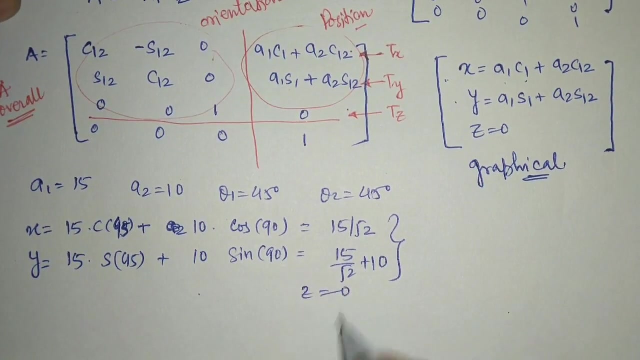 become 15 into sin 45 plus 10 into sin 90, and that will be how much 15 by root, 2 plus 10.. So that is my position. z is equal to 0 anyways, right, So we can say z is equal to 0 only.